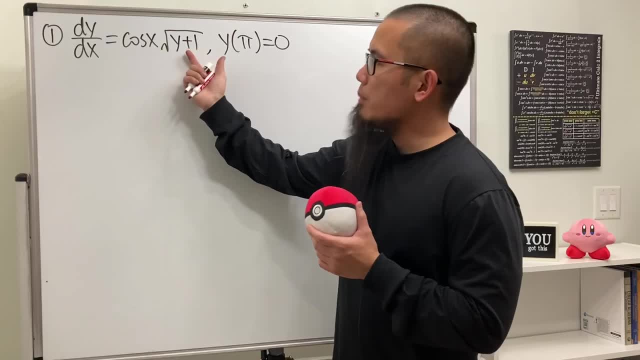 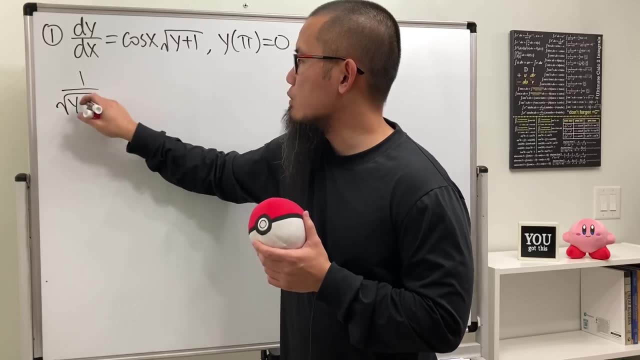 So you see, right here we have the square root of y plus 1.. We can put that to the other side by dividing this on both sides, So we get 1 over square root of y plus 1, which is the dy here. 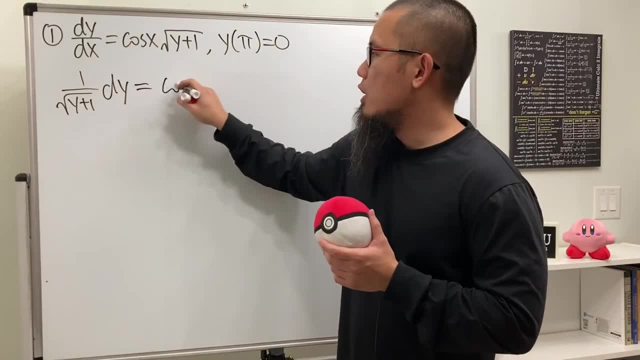 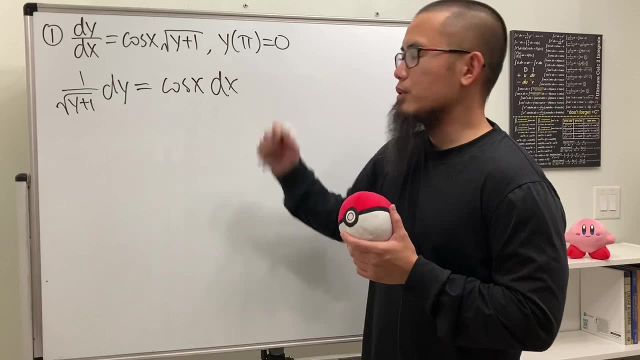 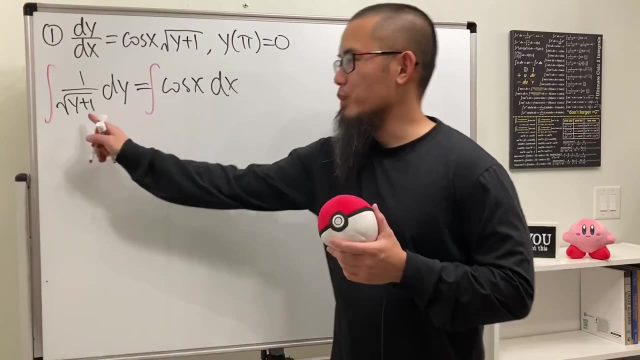 And then we can just multiply the dx on both sides. So we get cosine x- dx, like so, And you see y and the dy are together and the x and also the dx Together. So this is good, Because now we can just integrate both sides. How do we integrate? 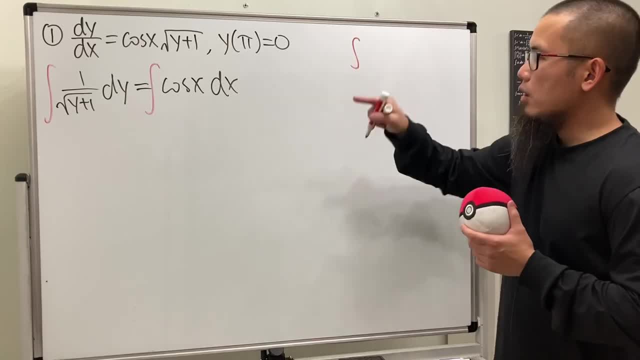 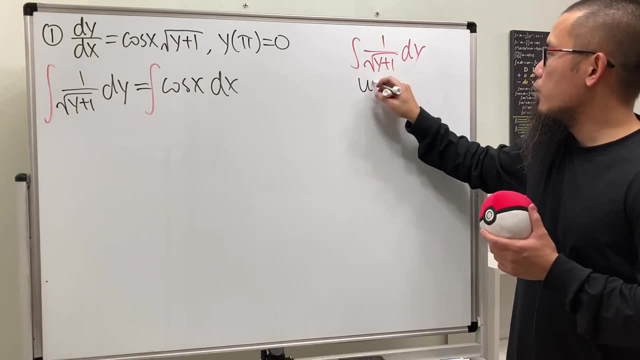 that. Well, let me show you guys on the side real quick, Integral of that 1 over square root of y plus 1.. We can just do a use of real quick. Let u equal the inside, which is y plus 1. And we see. 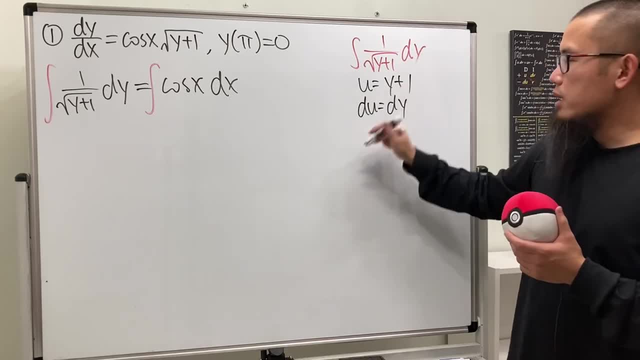 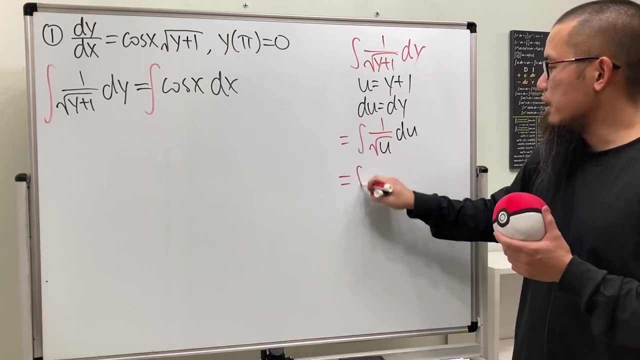 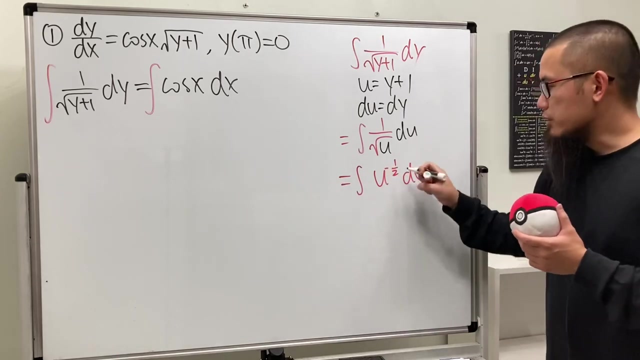 du is just the same as dy, And this right here is just the integral 1 over square root of u du, which is the same, Integrating u to the negative 1 half power in the? u world. Well, to integrate this, we'll just add: 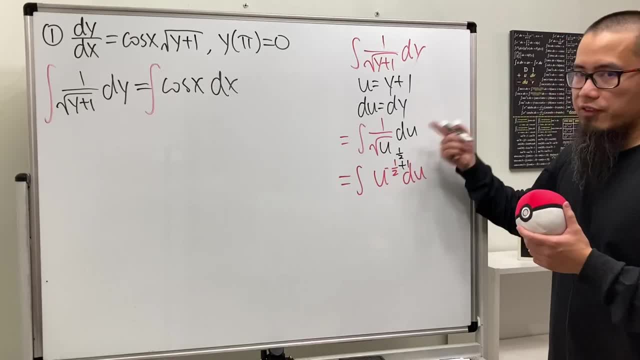 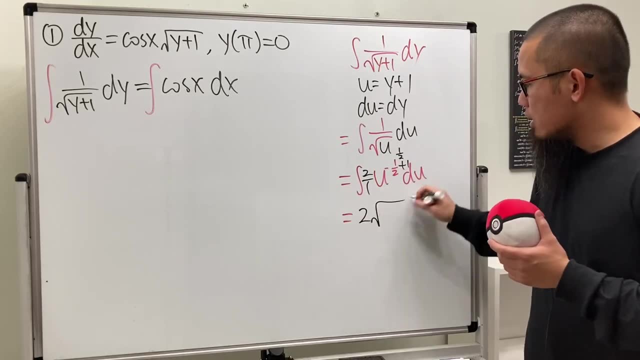 1 to the power, which will give us plus the 1 half, and divide it by the new power, which is the same as multiply by 2 over 1. And we will just get 2 times the square root of u, which is y plus. 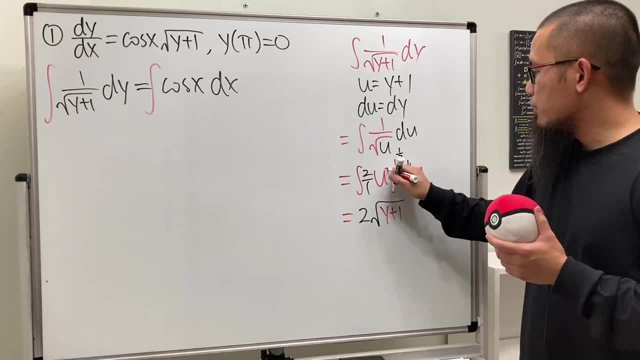 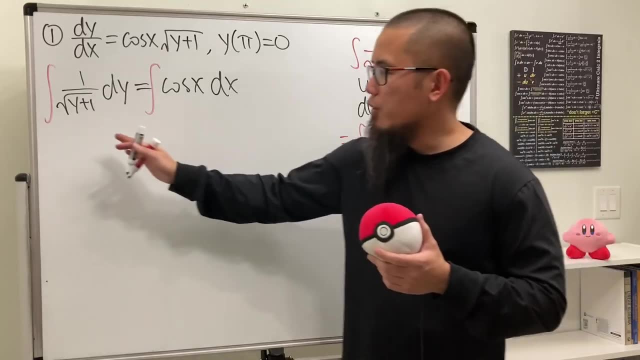 1. And right here you don't have to worry about the plus c. Technically you put on plus c here, but you also will put on plus c here. However, you can bring the constant from the left-hand side to the right-hand side. 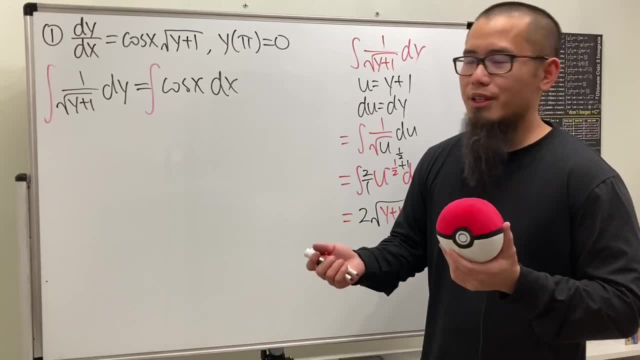 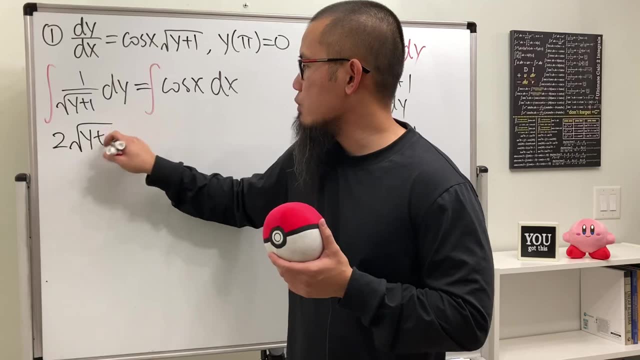 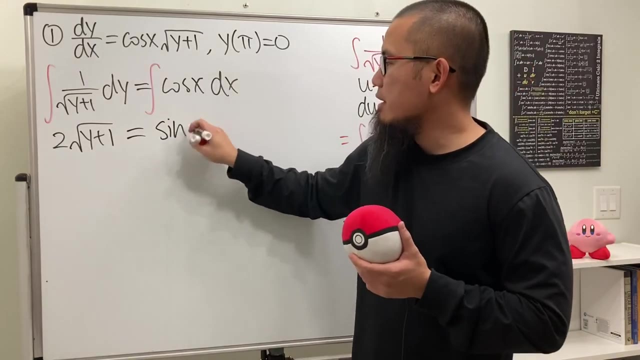 and the two constants together is still another constant. So I'm just going to write down the result right here, which is just that 2 square root of y plus 1.. No need for plus c, just do it on the right-hand side. Integrating cosine, we get positive sine. And then let's go ahead and 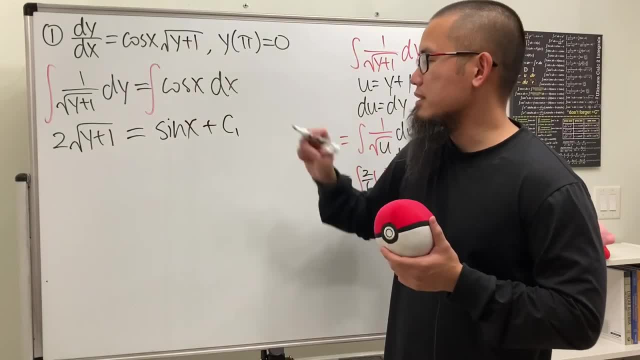 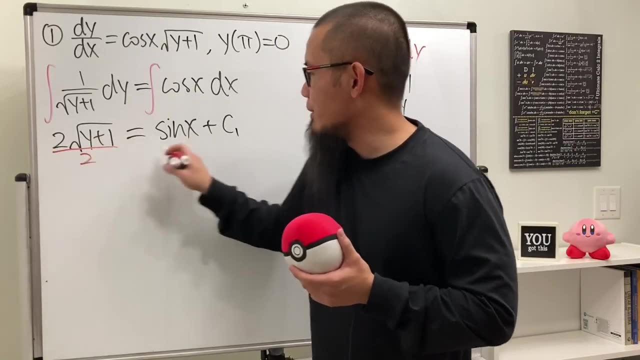 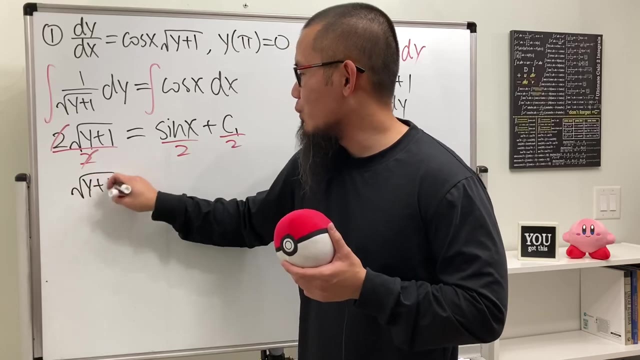 put down our constant. This is the first constant, so let's label that c1.. Because you will see, to isolate the y here, let's go ahead, divide everybody by 2.. I'm showing you guys, this step is because of this part right here, But anyway, we get square root of y plus 1 being equal to. 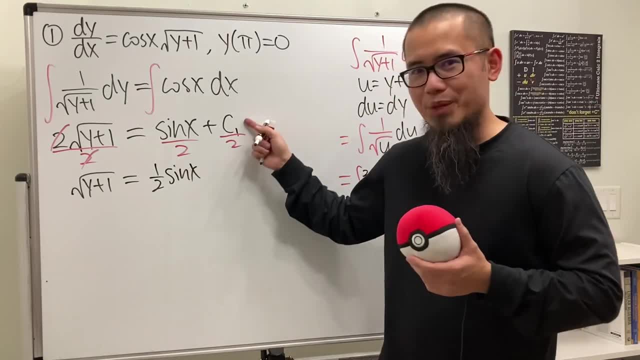 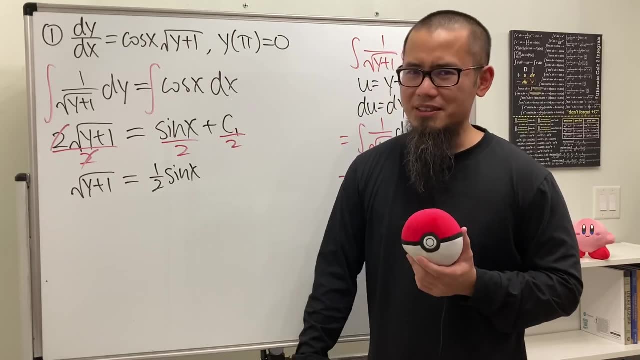 1, half sine of x. and then here we go. c1 is a constant, 2 is a constant, A constant divided by another constant is just another constant. So we are going to label this as c2.. Yep, And then. 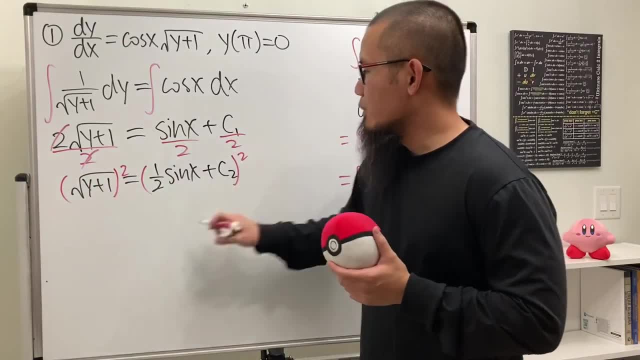 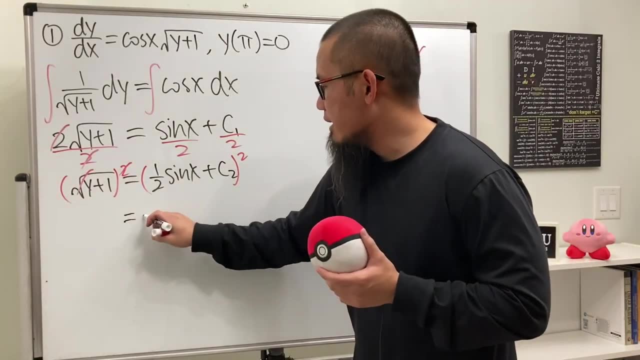 let's go ahead, square both sides, So you see this and that will cancel and this is going to be y plus 1.. We can put the 1 to the right-hand side, So we get negative 1 plus this thing, which is 1. 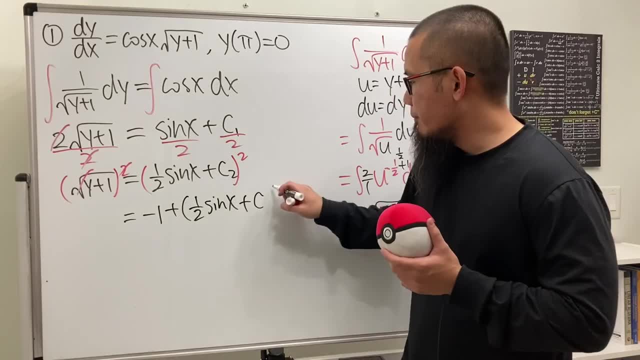 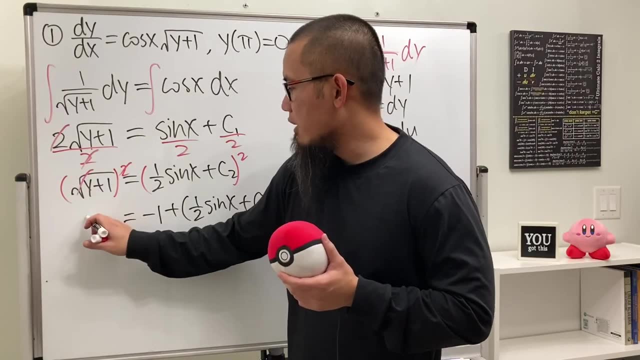 half sine of x plus c squared. And the reason I just write down c is because we are done. The left-hand side will just have the y by itself. Remember, the 1 is right here already. This right here is called the general solution. 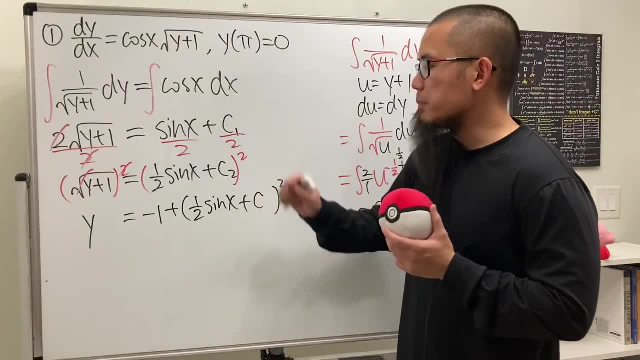 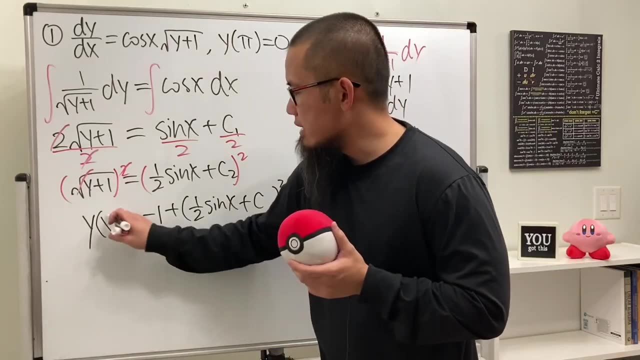 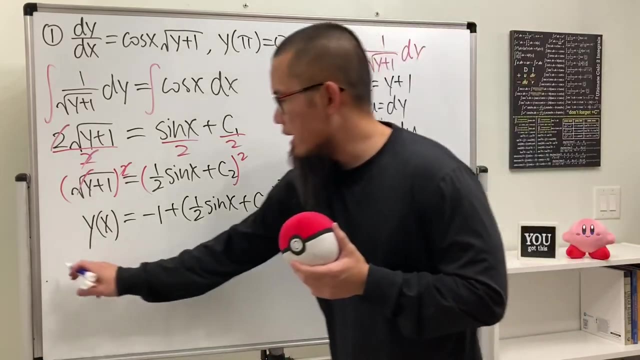 We can just present the answer right here with the c, without the subscript. Well, you also have to keep in mind that y is a function of x, So let's write this down: y as a function of x Now, because we have this initial value which says y of pi is equal to 0,. 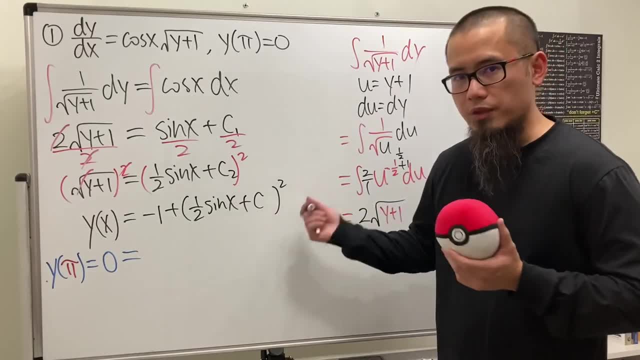 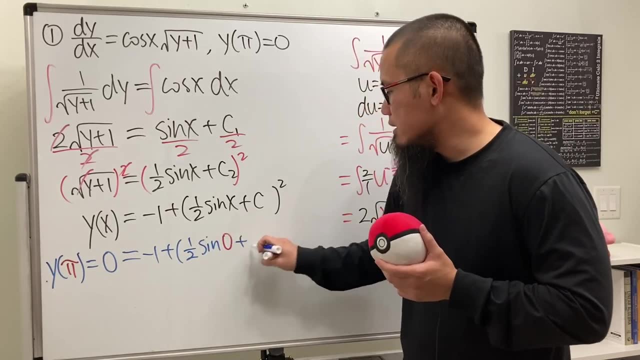 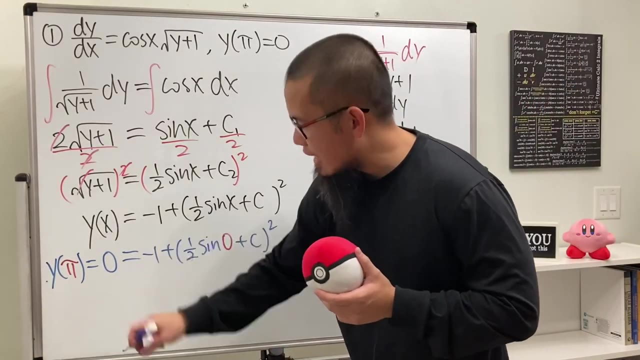 that means we can just put pi into this x here and then solve for c. So we get negative 1 plus parentheses. So we have y is 1 half times sine of 0 and then plus c and then square. Okay, look at this equation: Bring the negative 1 to the left-hand side, we get 1 equals. 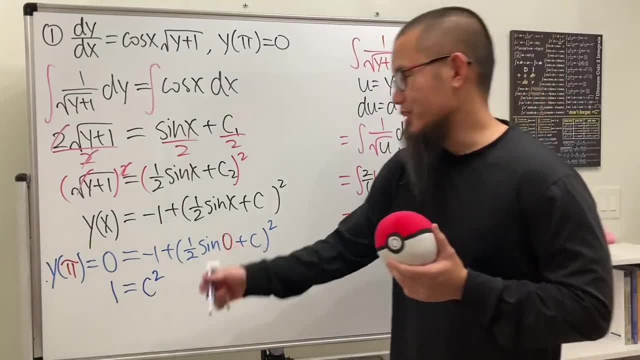 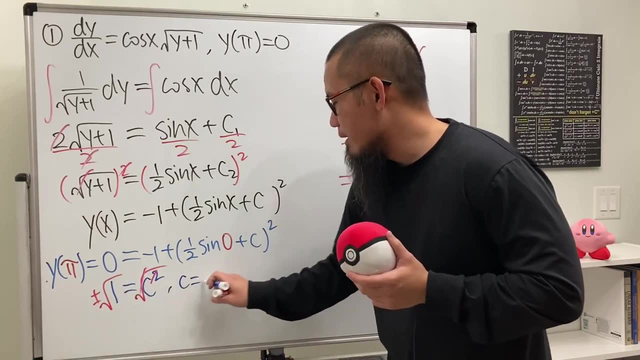 this is just 0, and then we have c squared. What's c? We'll do the square root on both sides And don't forget the plus or minus. So c is actually equal to plus or minus 1.. So in fact we have two answers. 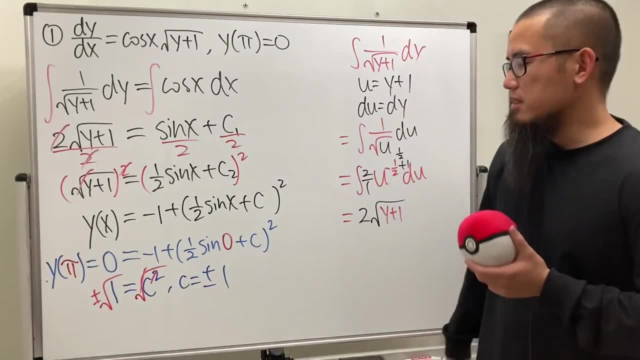 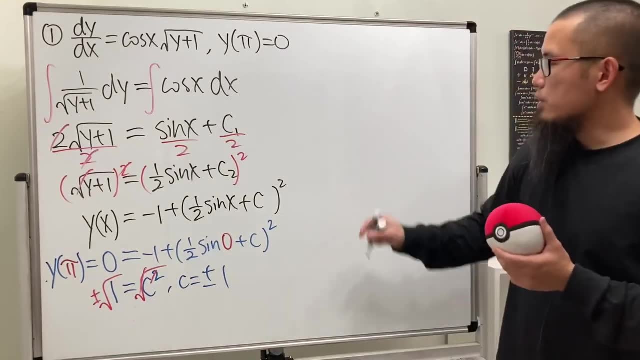 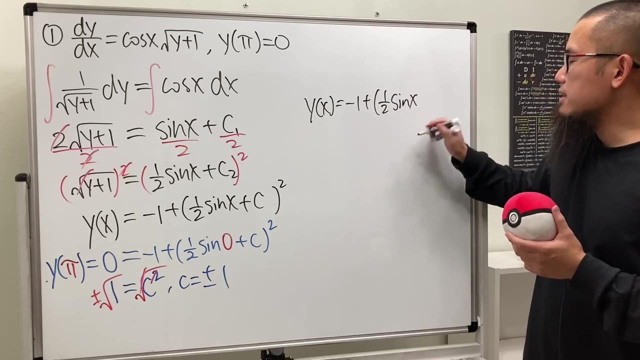 right, Because the first answer is with positive 1, and the second answer is with the negative 1.. So that will be pretty much it, and let me write down the final result for you guys. First we have y of x being equal to negative 1 plus 1 half sine of x, and then c is positive 1,. 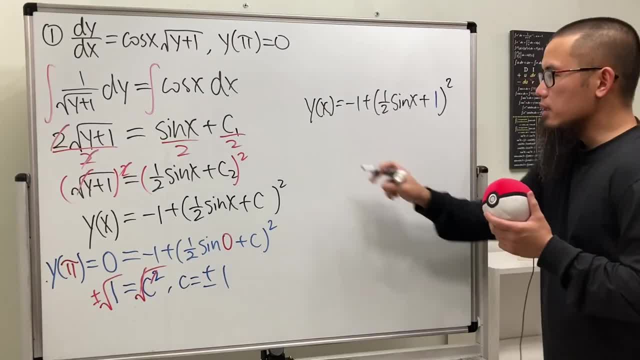 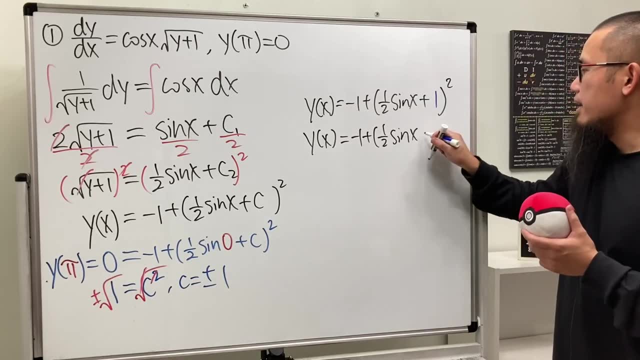 so we just add the 1 here and then we square The second one. we have y of x equals negative 1 plus 1, half sine of x and then minus 1, and then square This and that they will both satisfy the. 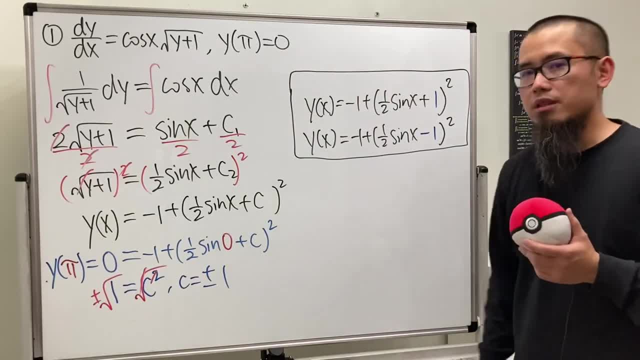 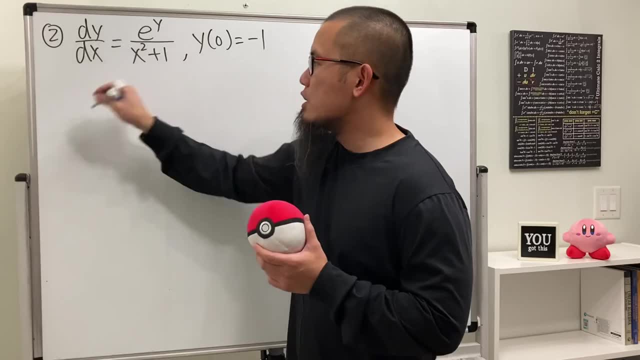 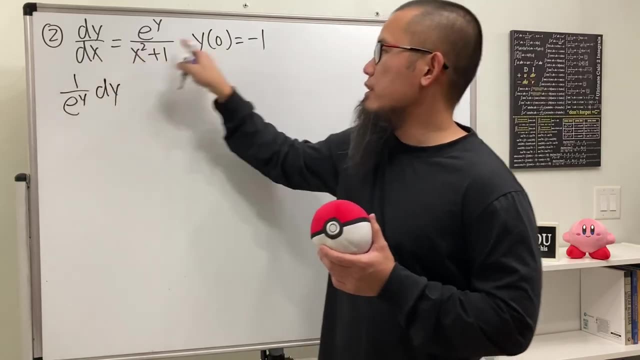 initial value problem. so they are both the answers. All right. here is our second problem. Well, we see that we have e to the y here. We can divide this on both sides, right? So we get 1 over e to the y on the left-hand side, together with the dy, and then, of course, we can bring this to 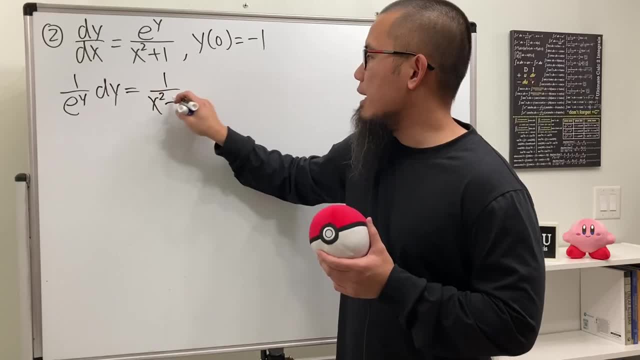 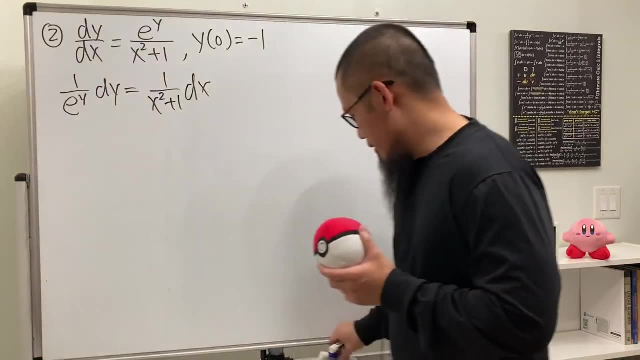 the right-hand side. so we have 1 over x squared Plus 1 dx, and now we can all be happy because we can just integrate both sides. So do it here, do it here, almost one color, Do it here, do it here, and then integrating this. 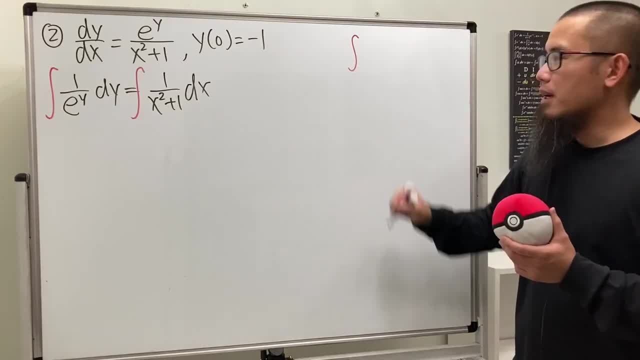 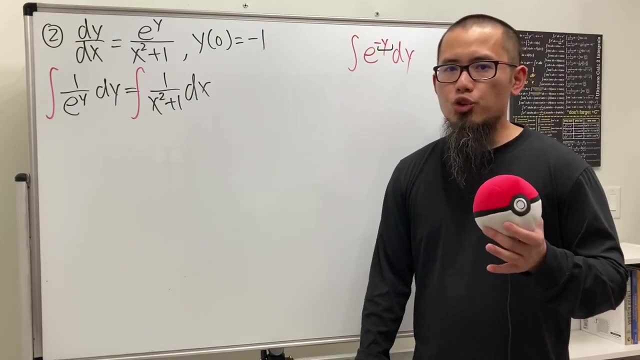 have a look here: e to the y on the bottom is the same as e to the negative y and of course you can do a u-sub real quick. let u equal that and you see du is just going to be negative 1. 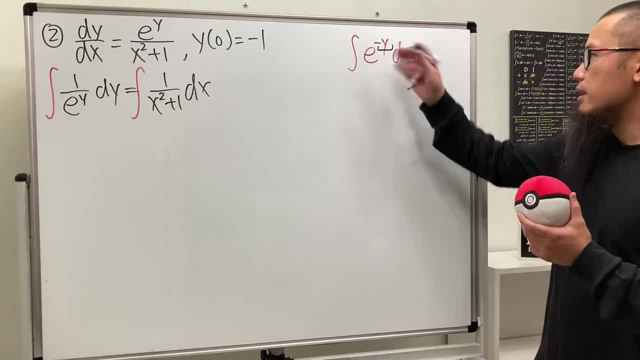 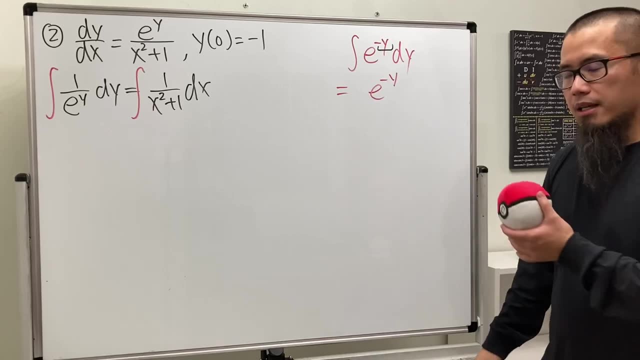 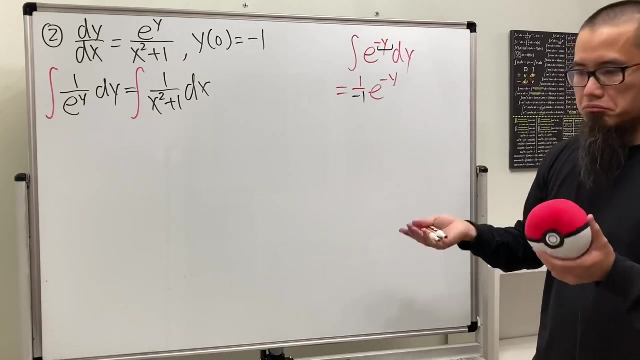 times dy. It's just a constant right, Negative 1.. So that's good, because this right here is just going to be e to the that power and divided by the derivative right here, which is the negative 1.. And you can do this whenever the inside function is just a constant. So this right 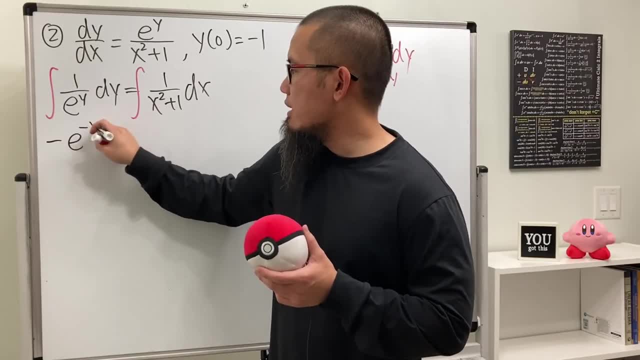 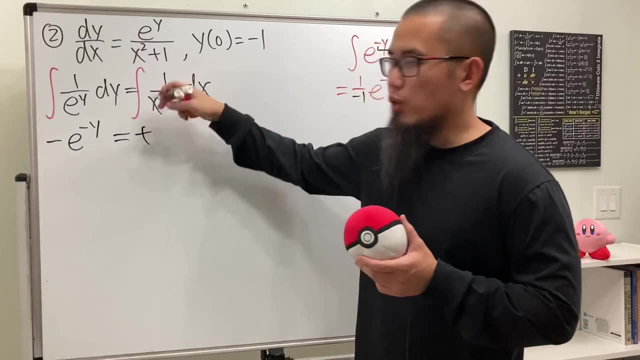 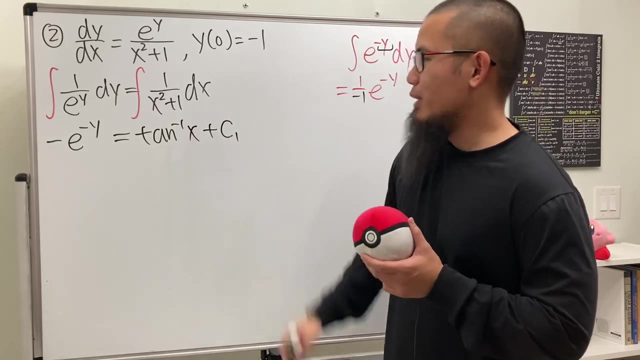 here is just negative e to the negative y, and then just put the constant on the right-hand side, So this is equal to the integral of this is inverse tangent of x. and then here we go plus constant And maybe that's already a c1.. Okay, here we have a negative, so perhaps let's divide everybody by. 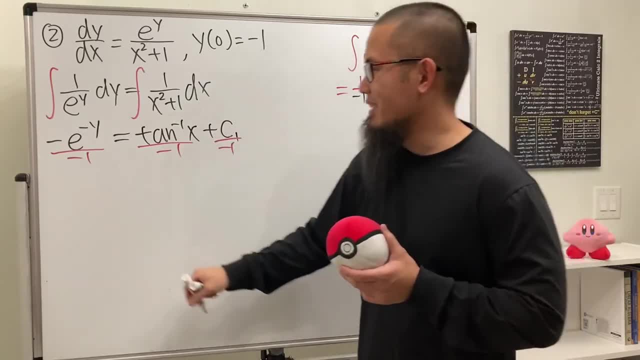 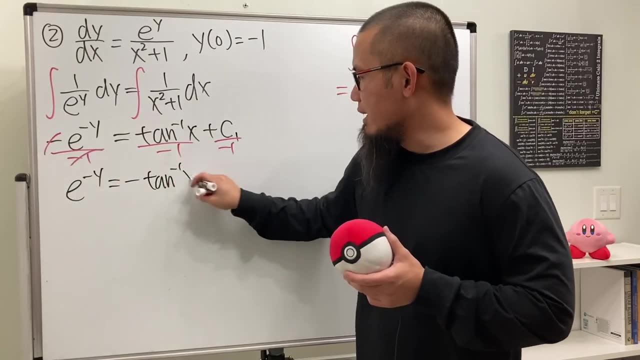 negative 1.. This is a lot of fun, right here, right, And then cancel this out and we get e to the negative, y being equal to negative inverse tangent of x. Here we go. c1 is a constant negative, 1 is: 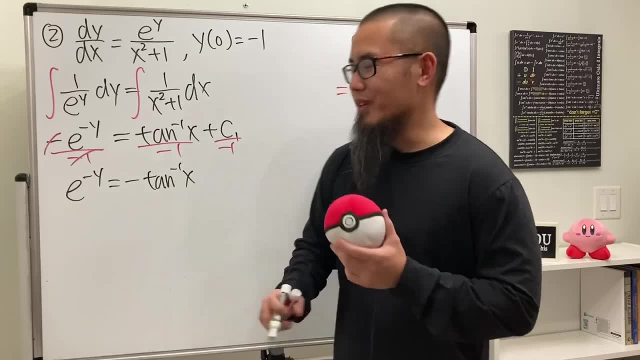 a constant. When they divide, you just get another constant. so therefore, let's just put down plus c2.. How cool is that? Okay, I want to solve for the next problem. So let's solve for the next problem. So let's solve for the next problem. 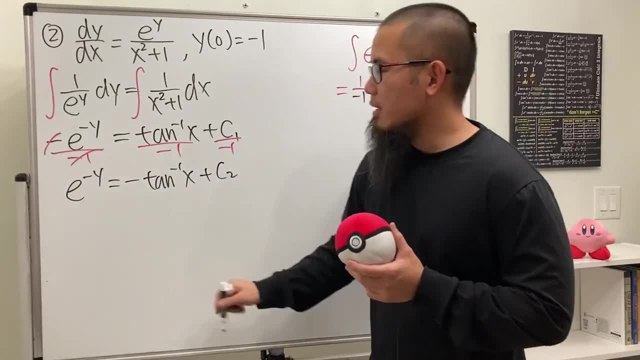 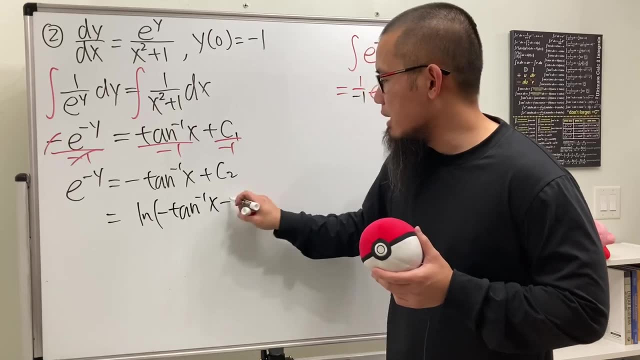 Okay, I want to solve for the next problem. So let's solve for the next problem. So let's solve for the next problem. the y right here. first we take the natural log on both sides so we get ln of the whole thing inside. so negative inverse tangent of x plus c2 that will give us negative y so we can divide. 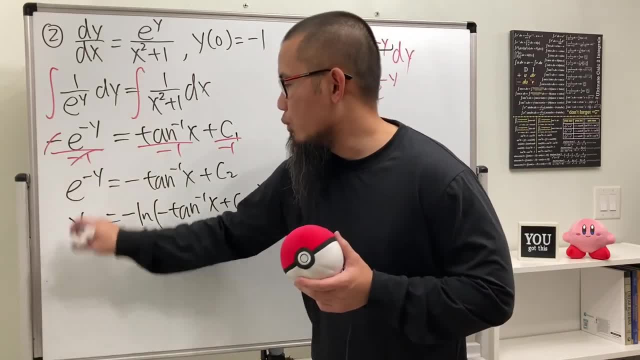 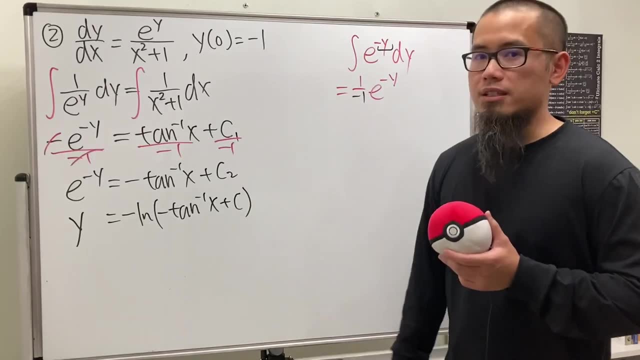 the negative on both sides. so we make this negative and then we can get y by itself. that's pretty much it so, in fact, here i am just going to label that as c. we don't need a subscript anymore. and then, right here we can write this: y as a function of x. 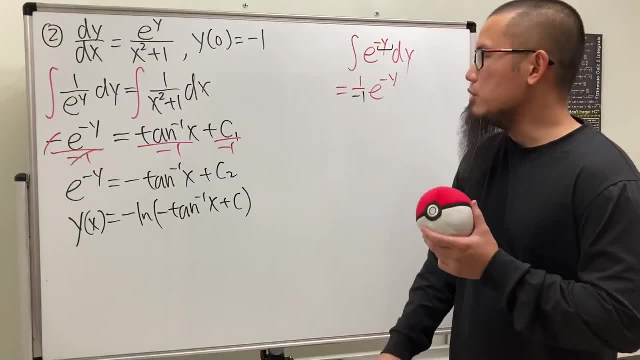 we don't need a subscript anymore. and then, right here, we can write this y as a function of x. we don't need a subscript anymore. and then, right here, we can write this y as a function of x. now we have this initial condition: y of zero is equal to. 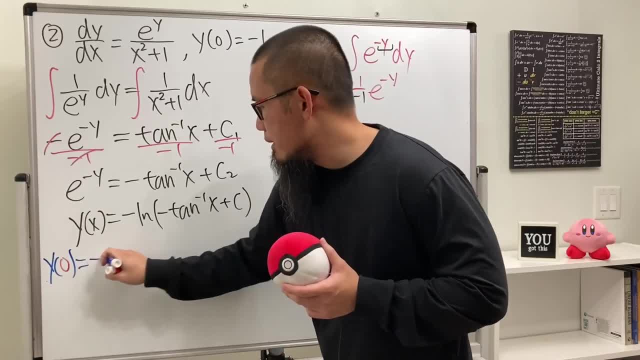 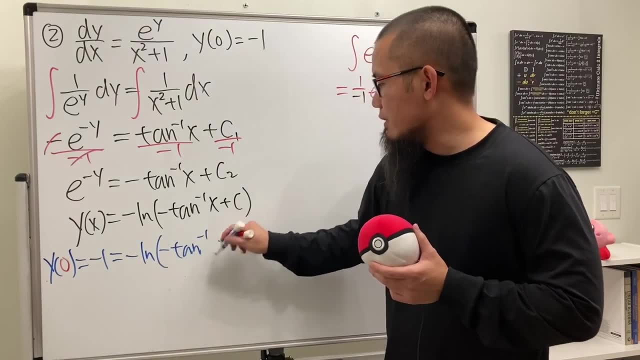 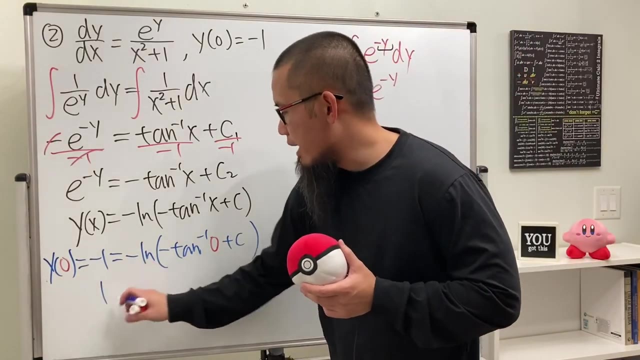 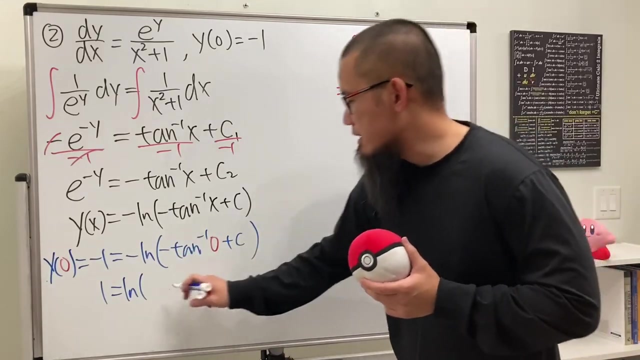 one, sorry, negative one. and uh, we have the right hand side, that's negative ln parentheses: negative. inverse tangent of zero plus c. have a look: negative, negative. so we just get positive. one equals positive ln. inverse tangent of zero is zero. multiplied by negative is still zero. so inside here is just c? ln of what will be one. e right, you can just do e to this. 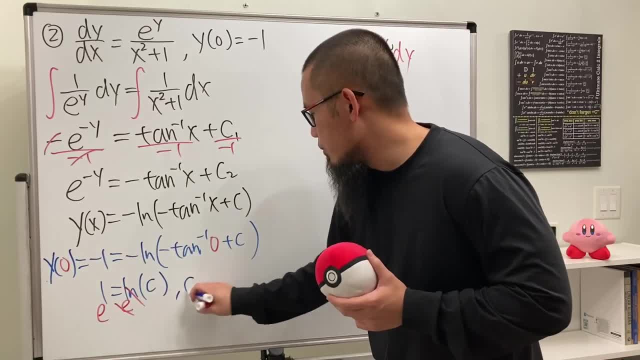 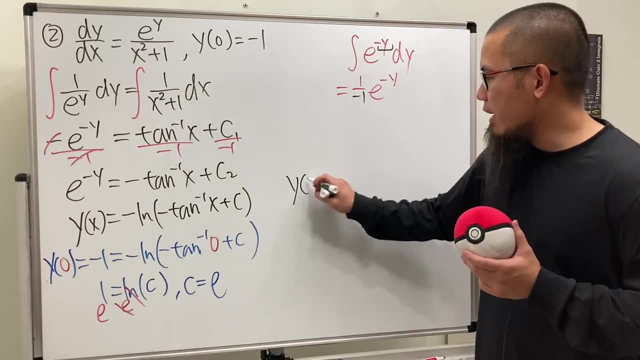 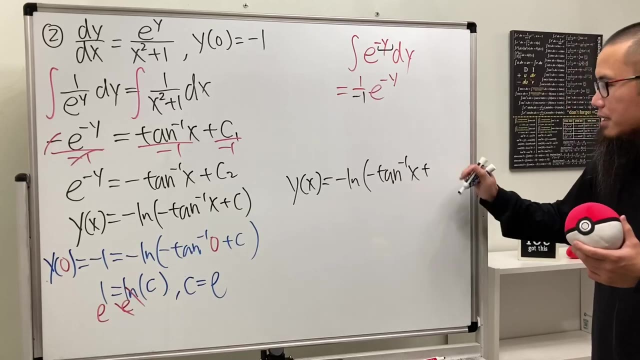 power, e to the power, if you like, and then we get: c is equal to e. a lot of letters, all right. so we are done pretty much. so we get y of x being equal to negative, ln of negative inverse tangent of x, and then plus not c, but rather we have e. 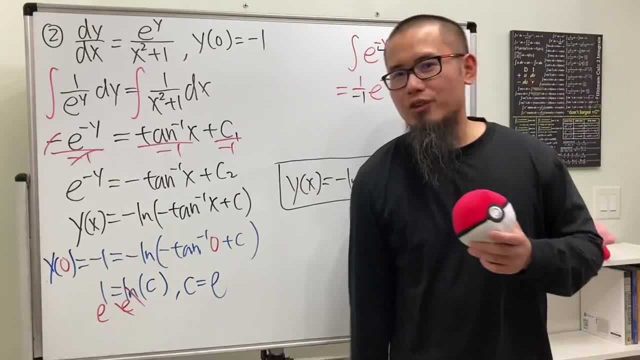 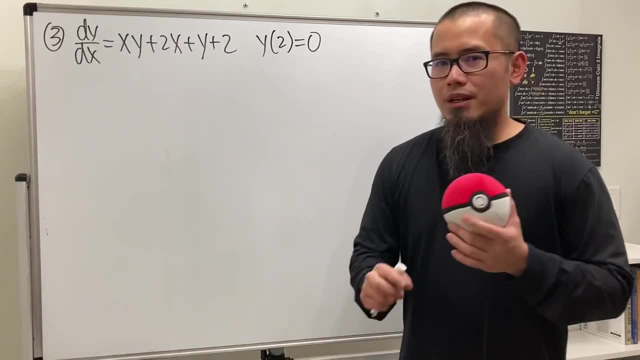 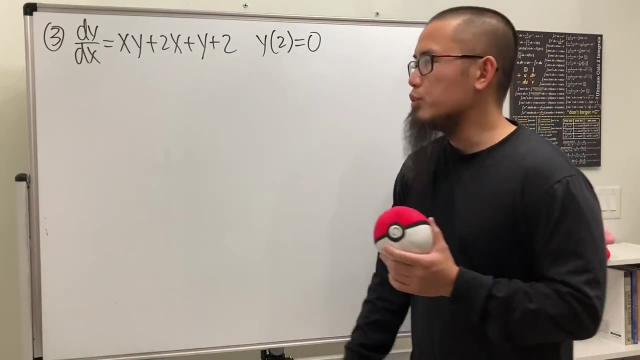 and then here is the solution to that initial value problem. okay, take a look at number three. right here we have dy. dx is equal to all this. be sure you do not minus the y on both sides, minus the x one by side. no, don't do that. what we will have to do is look at the right hand side and 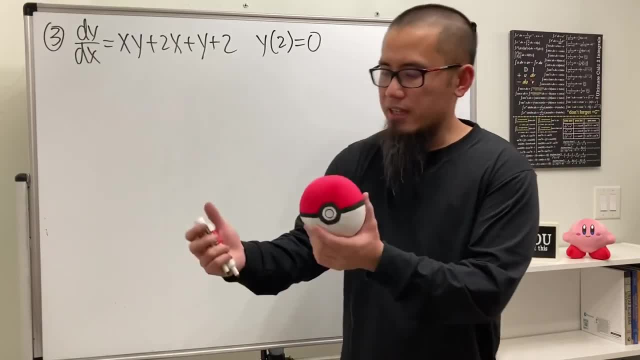 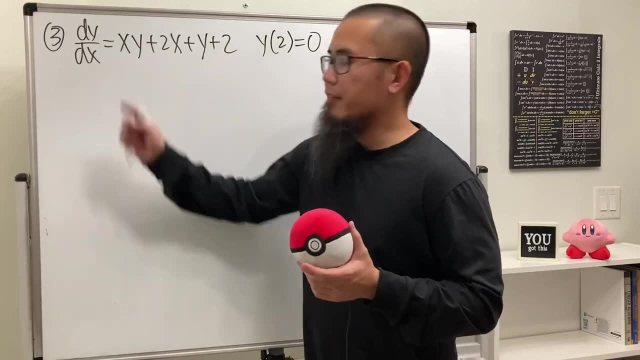 then try to factor it and hopefully we have a factor in terms of just x and then the other factor in terms of just y. let's see if we can make that happen. we have four terms right here. do the google business, namely factor by grouping. look at this and look. 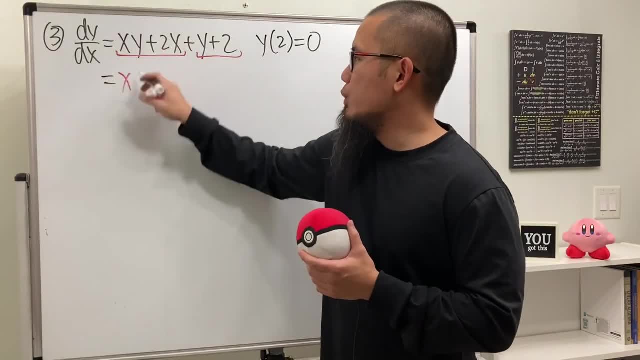 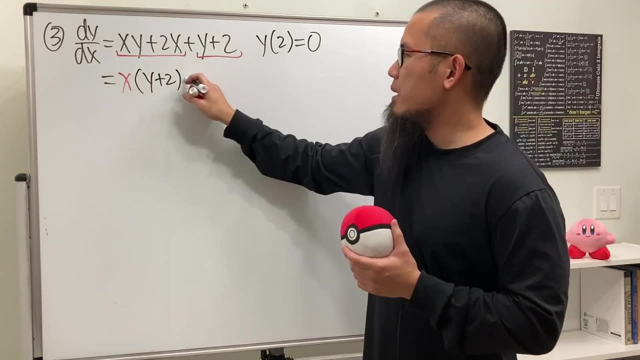 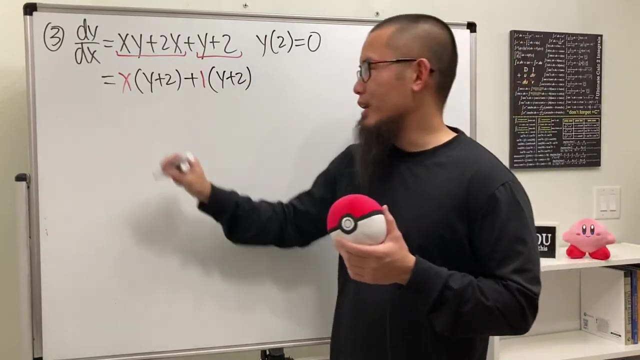 at that: well, this and that we can factor on x and then we will get y plus two. that's really good, because you see this is also y plus two, but right here, technically, you can say plus one factor of one, and then we have the y plus two. if you look at it this way, you see that 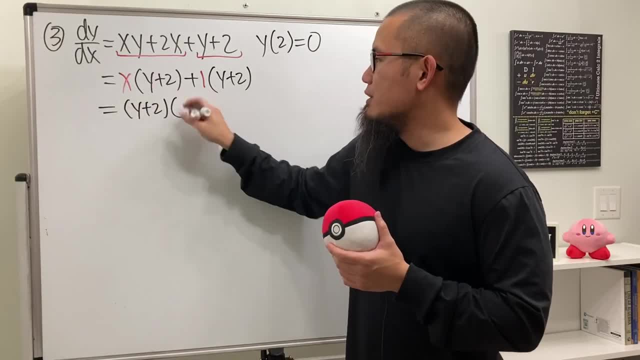 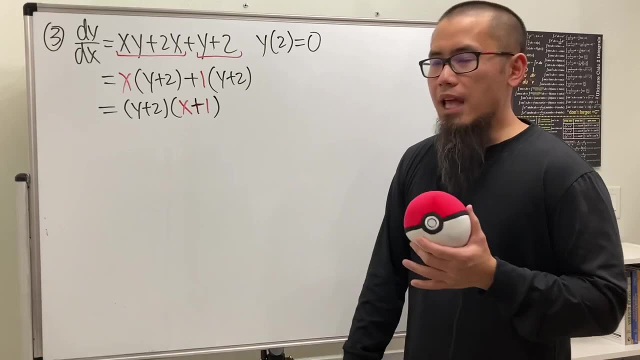 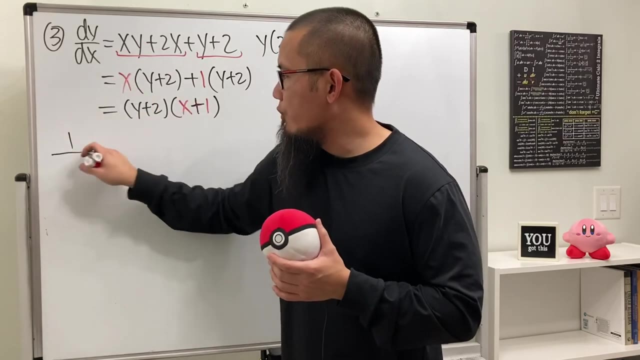 we can factor out the y plus two, and then the other factor is just x plus one. very nice, huh, and perhaps i'll just match the color right here. and now we have dy. dx is equal to that. we can just divide this on both sides, so we get 1 over y plus 2 with the dy, and that. 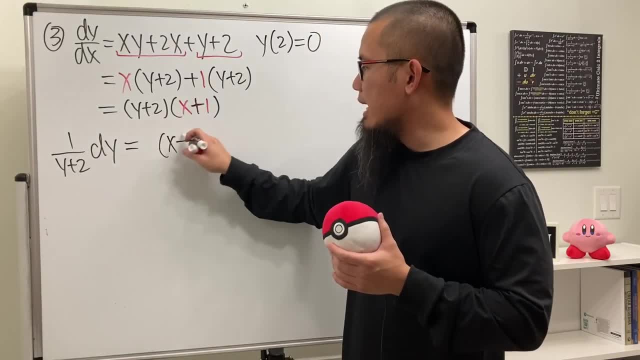 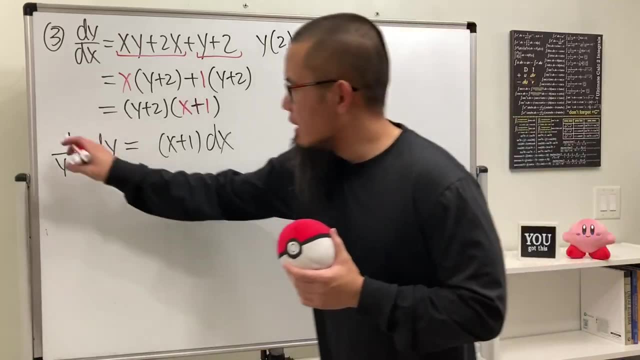 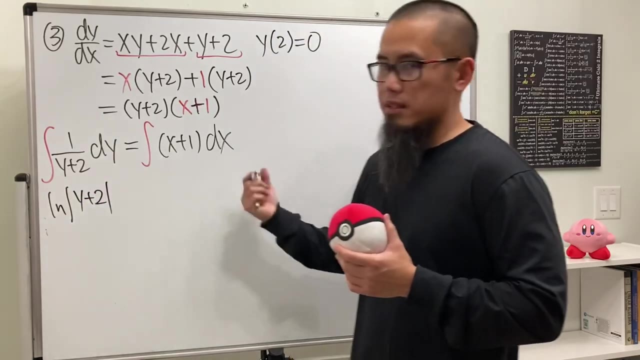 will be equal to this right here, still on the right hand side, and then let's bring the dx right here. aha, we can then integrate both sides. do it here. do it here on the left hand side, we get ln value of y plus 2, and again c will just be on the right hand side. integrating this, we get 1 half. 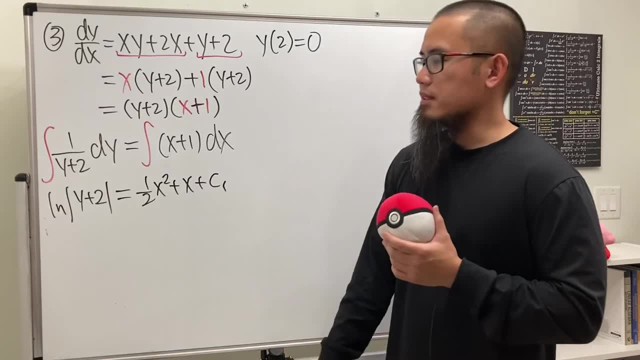 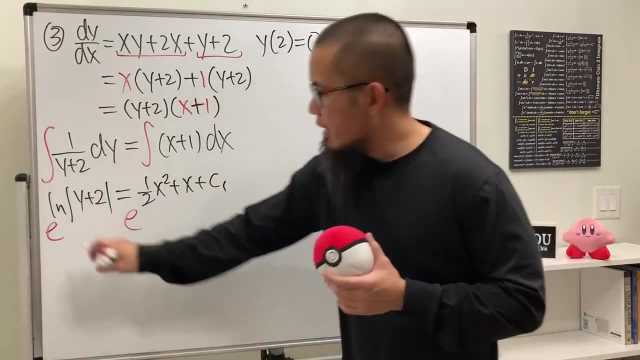 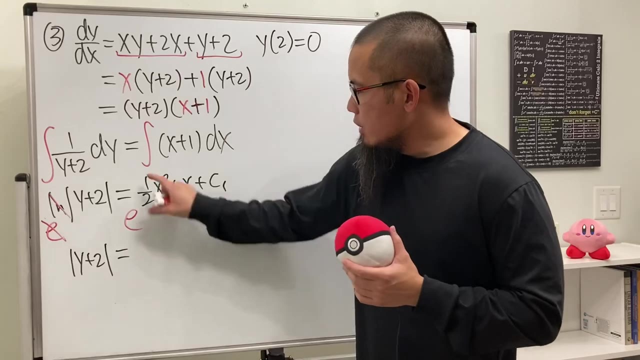 x squared plus x, and here we go. this is the constant. now to get the y by itself, let's do e to that power and e to the whole thing, right here. cancel, cancel, and then we have absolute value of y plus 2.. check this out: e to this power, and they are all adding. i'm going to break it down as e to: 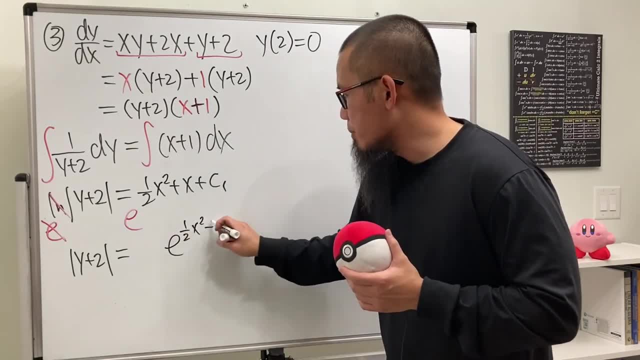 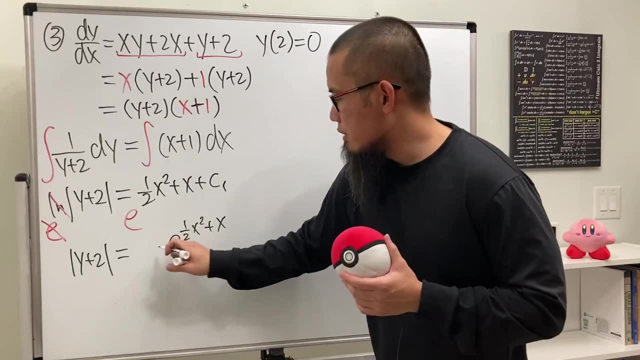 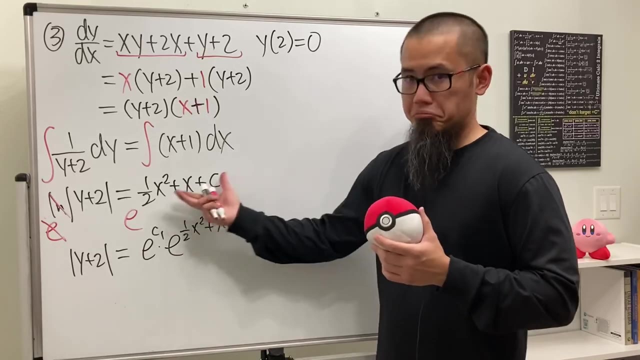 that down, which is e to the one half x squared plus x. that's just the function part, and then i'm going to look at e to the c1 right here. so i'm going to say e to the c1 and of course, if you look at it backwards, this times that you just add the exponents. so that's what we have. 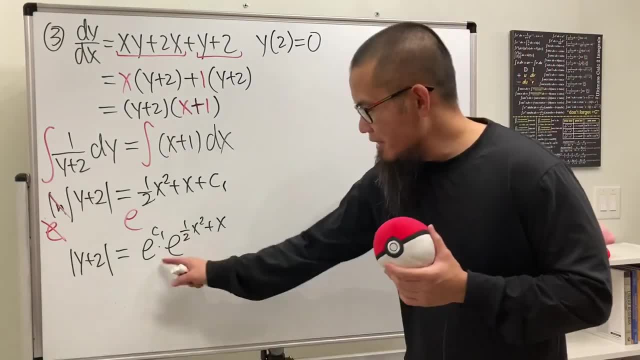 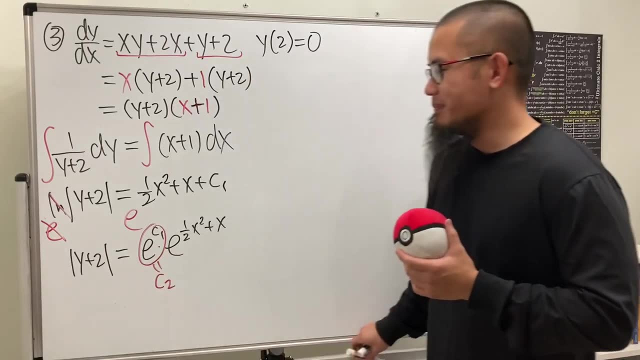 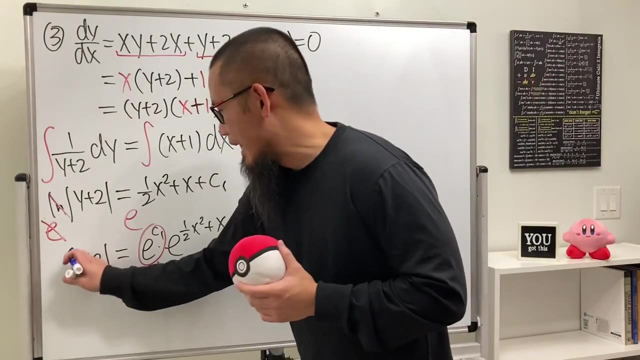 here we go. c1 is a constant, e is a constant. a constant to a constant is just another constant. so we are going to look at this and label that as c2. all right, now let's think about how we can get rid of the absolute value. you literally just get rid. 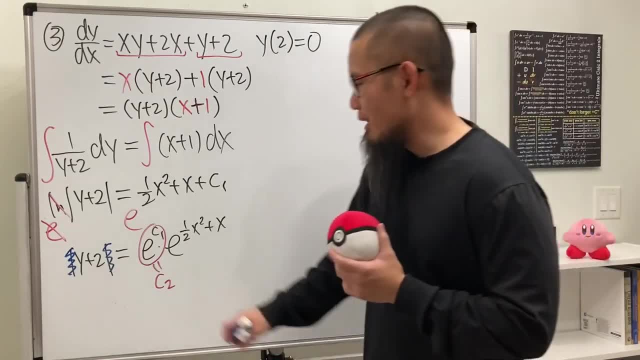 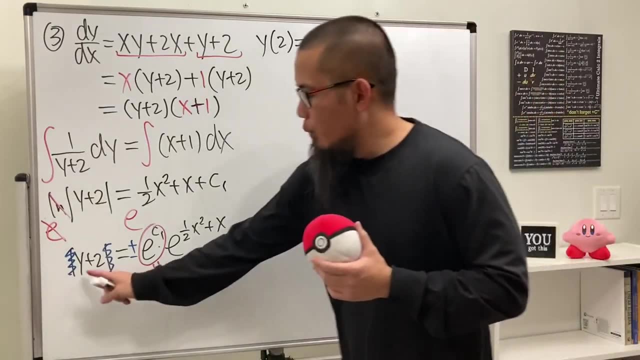 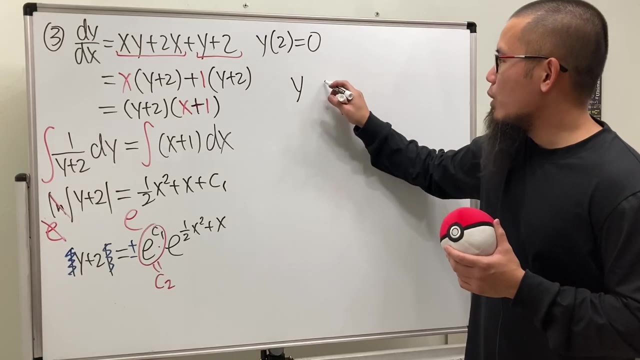 of the absolute value, but you will have to put plus or minus on the right hand side. okay, that's pretty good, and now i'm going to write down the work right here we have y plus 2. we can put a 2 to the right hand side, so we get y by itself now, and then that will be equal to negative 2. 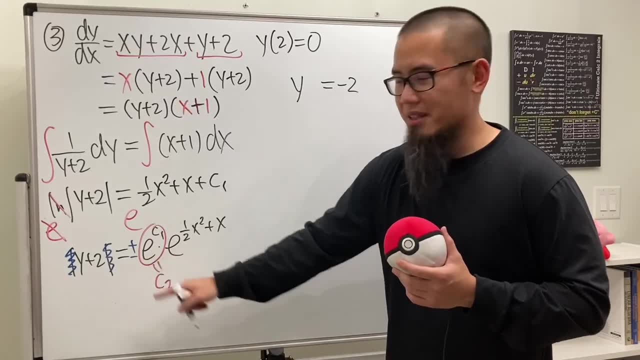 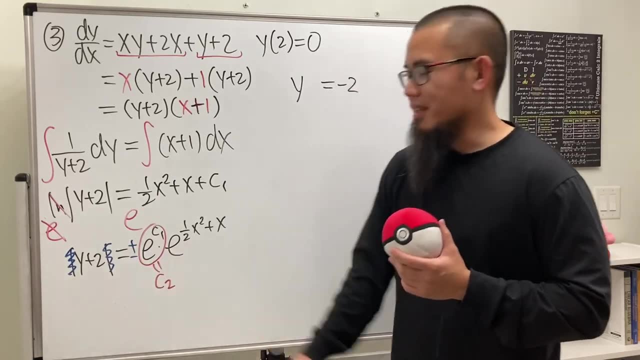 let's put a 2 to the other side. here we go again. this was labeled to be c2 earlier, but you see, positive c2 is a constant, negative c2 is enough, it's just a constant. so together we're just going to label that as. 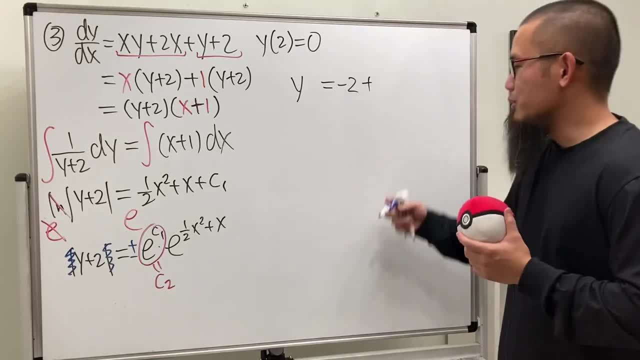 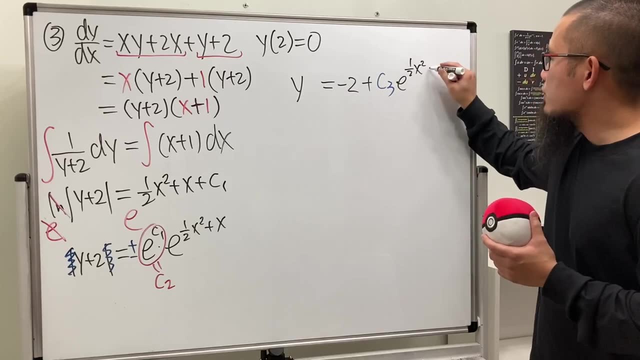 c3. so i'm just going to say plus c3, and then we have e to the power. so let's just write that down: e to the 1 over 2, x squared plus x, and because we got the y by itself, we don't need to have the 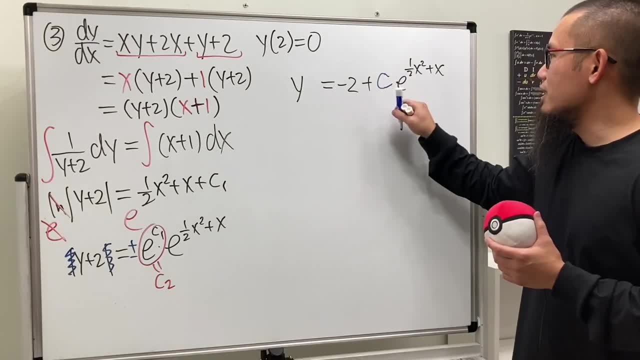 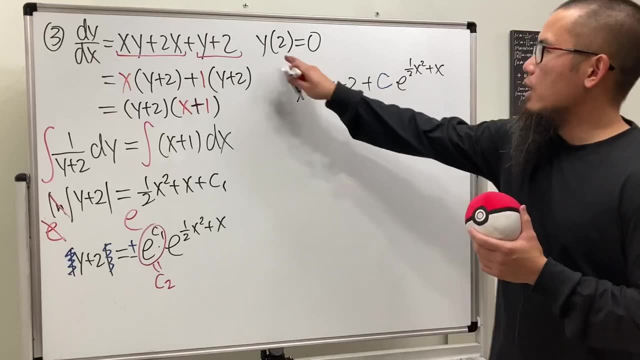 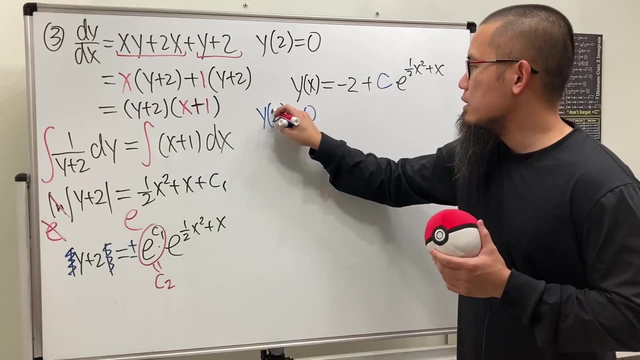 so this right here will be our c for the general solution. let's make it slightly bigger. and we know this is y as a function of x. okay, we know this right here. so let's go ahead and solve that. so y of 2 is equal to 0 and this means x is equal to 2.. plug in here so we get. 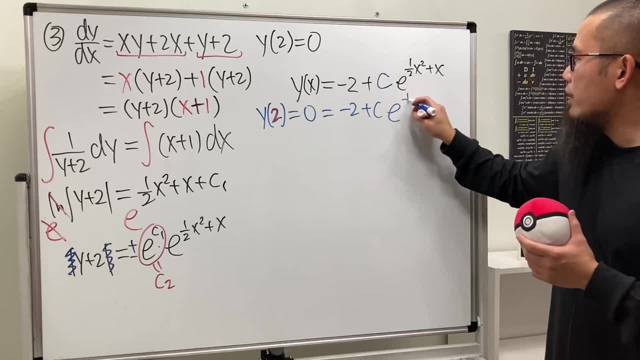 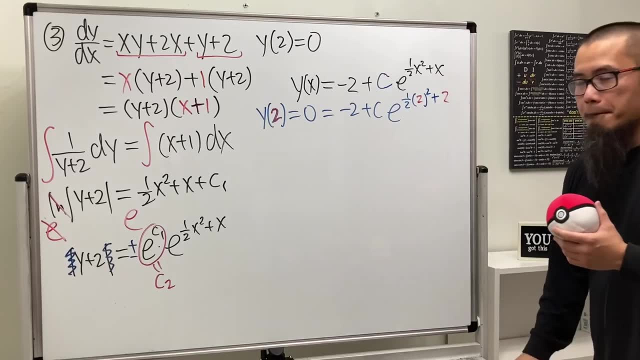 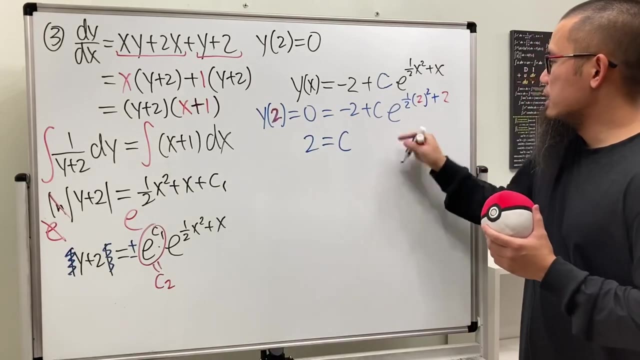 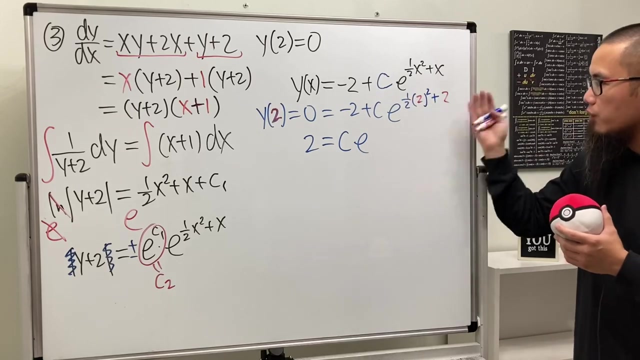 negative 2 plus c and then do e to the 1 over 2 times 2 square and then plus 2 power. like that, let's bring the negative 2 to the other side. we get 2 is equal to, and this is c and this is e. check this out. this is going to be 4 divided by 2 is 2. 2 plus 2 is 4. 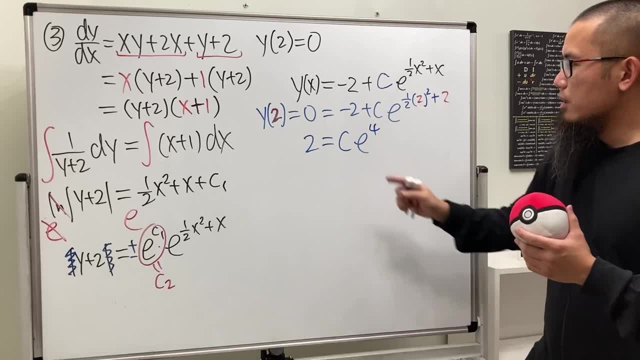 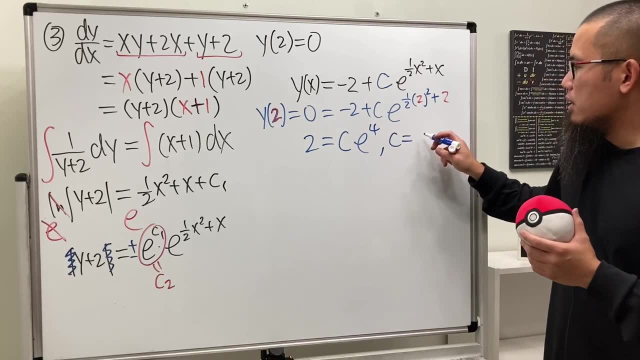 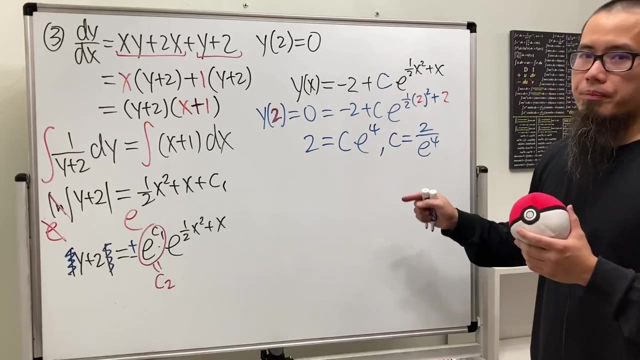 so this is e to the fourth power. okay, so how do we get the c divided? e to the 4 on both sides. so you see that c is just going to be 2 over e to the fourth power. so we can then put this back here. ladies and gentlemen, we are looking at y of x. 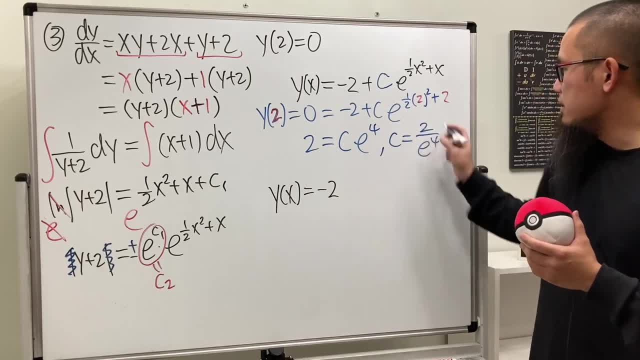 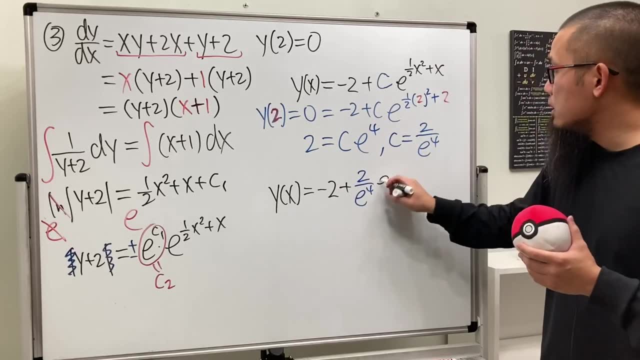 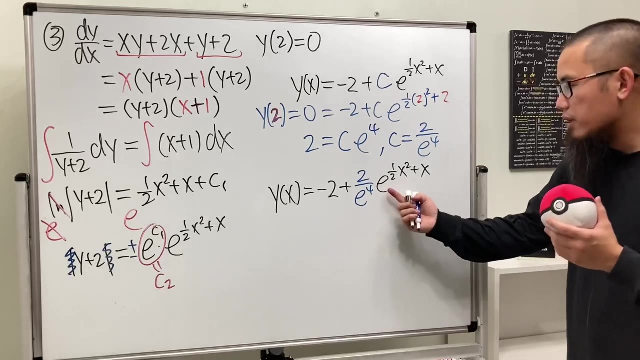 being equal to negative 2, and then the c is that which is plus 2 over e to the fourth power, and then we have all that which is e to the 1 over 2, x squared plus x- but you see this right here- has the base e, likewise that. so perhaps we can just do this power. 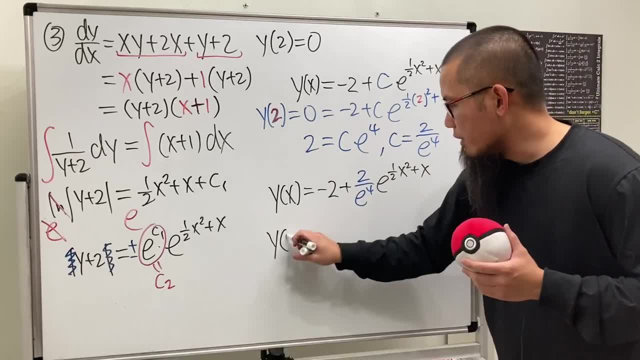 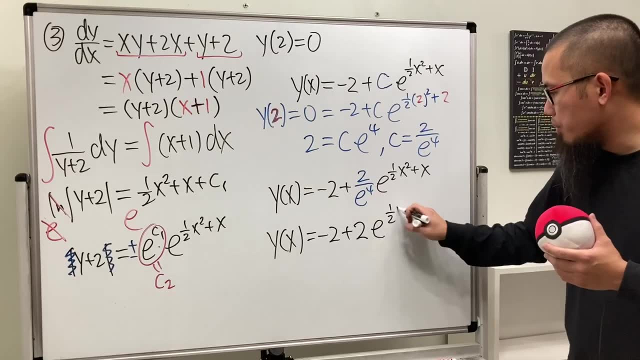 minus that power. so i'm going to write this down: y of x being equal to negative 2, plus just a 2 right here, and then e to the 1 over 2 power times x. e to the 1 over 2 times x squared. 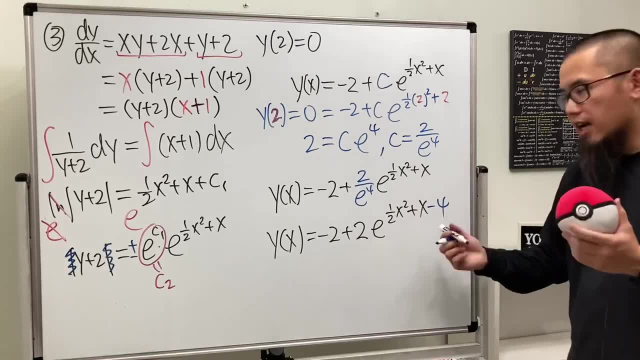 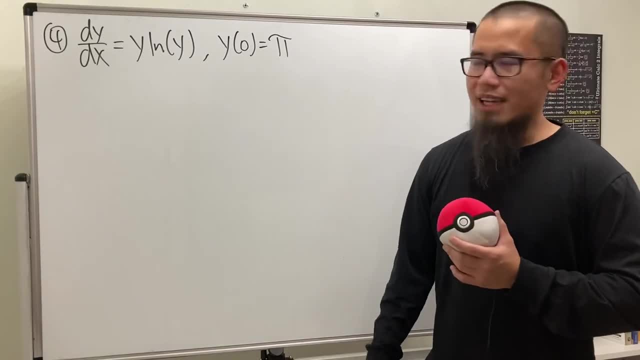 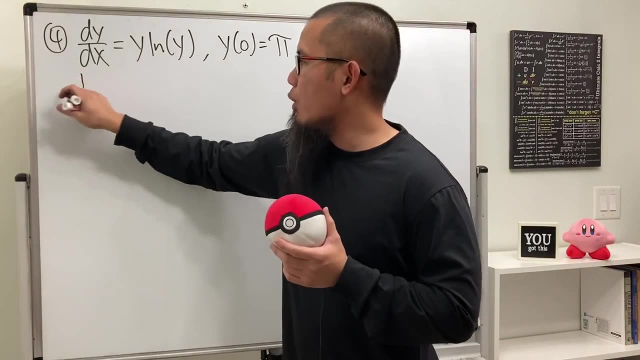 plus x and then minus the 4.. yeah, just like this. okay done. i like number 4 a lot. check this out: divide the x is equal to y times l and y. divide this on both sides, we get 1 over y, ln, y and then we have the dy here and that's equal to dx. 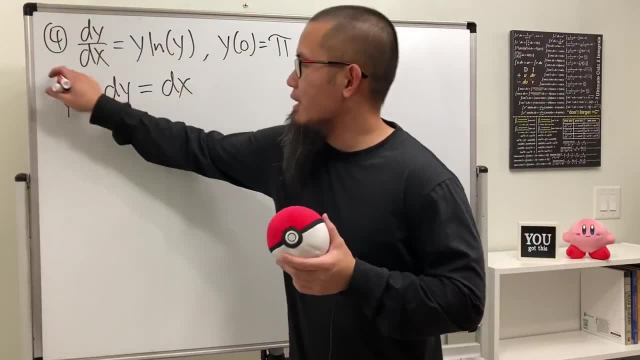 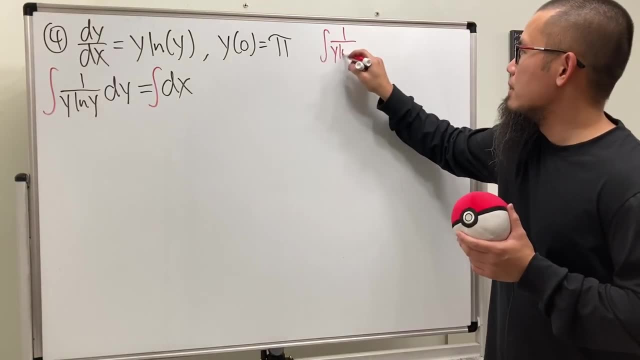 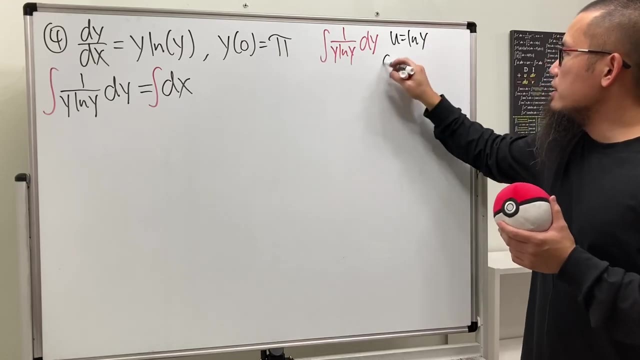 and then the different, not differentiate, integrate both sides, of course. integral, integral, integrating different side. we get what? now, let's do it on the side, we can just do, use up. let's do it together right here. let u equal l and y, so let's go ahead and make that happen. differentiating this, we get. 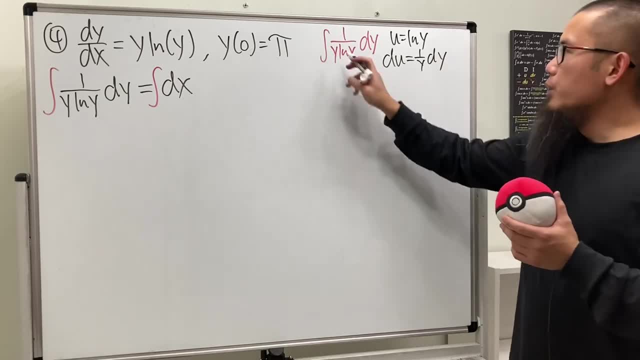 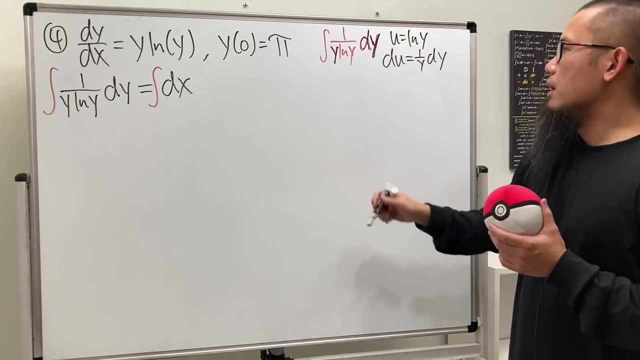 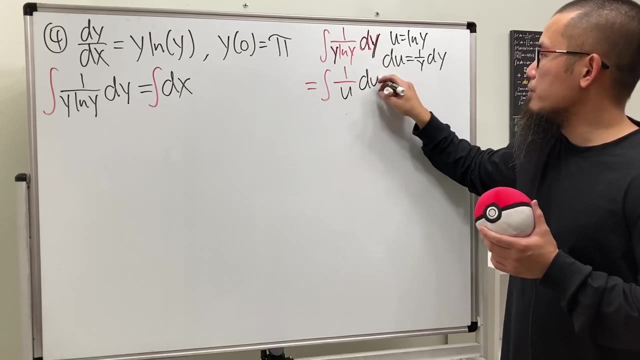 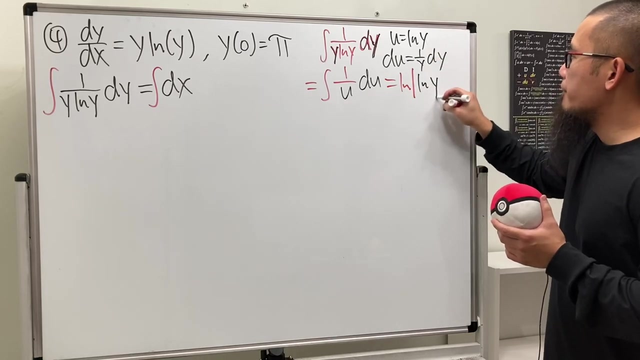 u equals 1 over y dy, and we have that right here, right, 1 over y and also the dy. that's so good. and you see, this is just integral. 1 over this is the u, and then the rest right here produce the du. so this right here will give us ln, x, Lu of u, which is that l and y. cool. so on the left hand side, 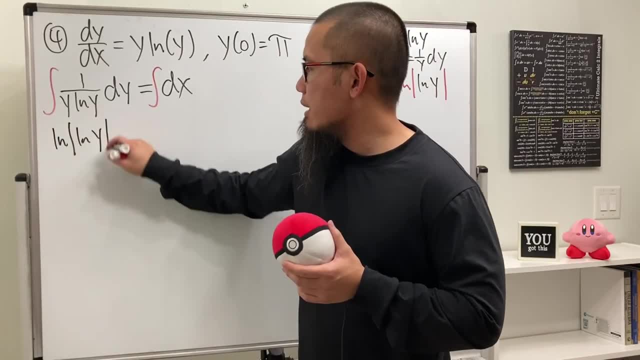 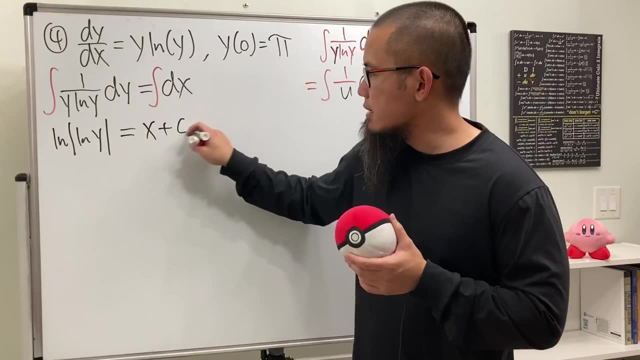 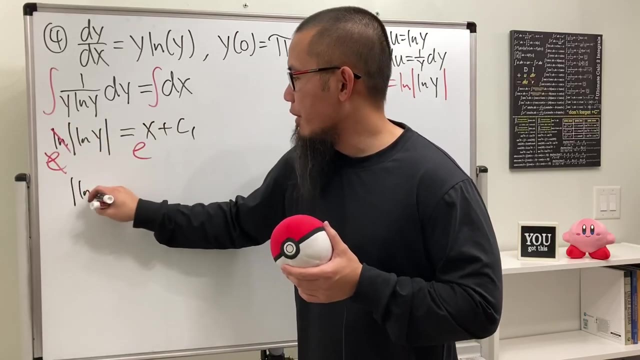 we get ln, the value of l and y. don't worry about the constant, just put it down on the right hand side. integrating dx, we get x. and then here we go, plus c1. here we go: e to the power. e to the power, cancel, cancel, abs. the value of l and y is equal to e to this power times. e to the power. 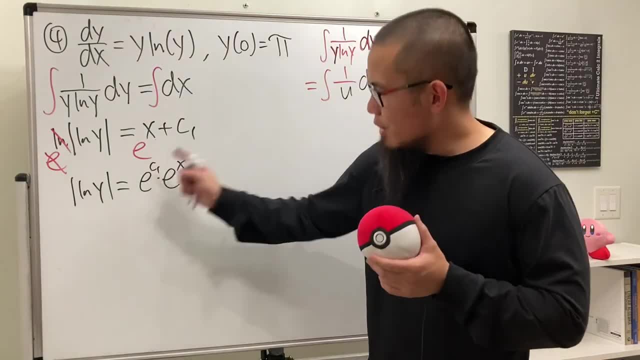 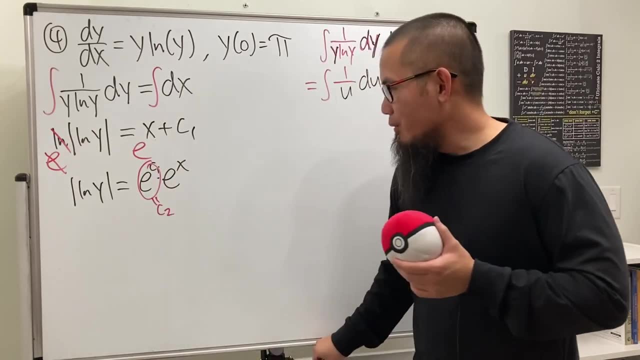 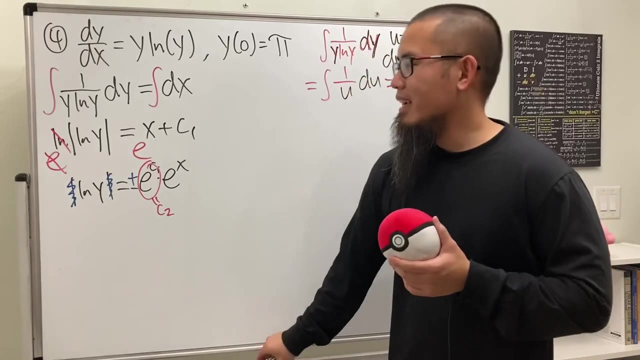 here we go. c1 is a constant, e is a constant. constant to constant is just another constant, so let's label this as c2, all right, and then we are going to get rid of the absolute value and remember we will have to put down plus or minus, and we see that the left hand side gives. 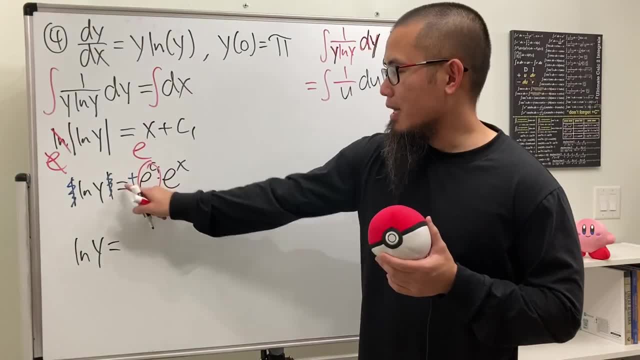 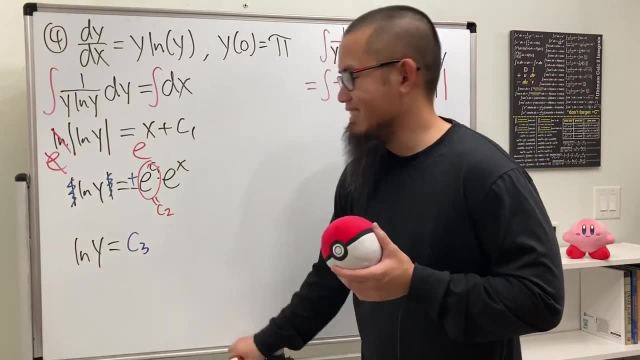 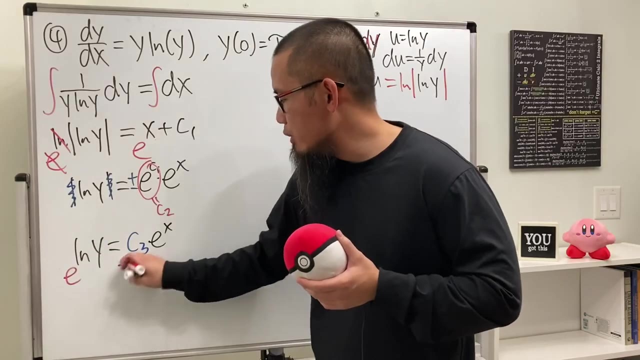 us l and y, and here we have plus c2, which is a constant. negative c2 is a constant, so let's just label that as c3. and then we have e to the x- cool, and now we will just do e to the power, e to the power again, cancel, cancel. so we get y by itself, and then on the 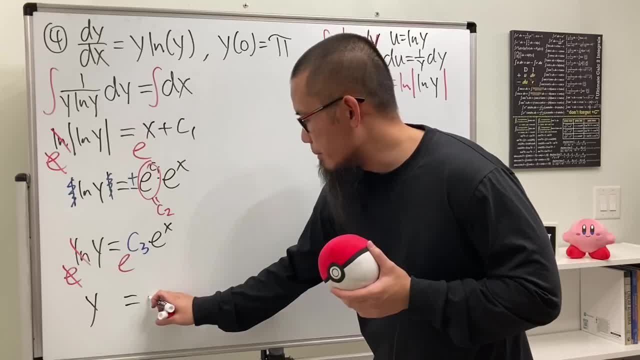 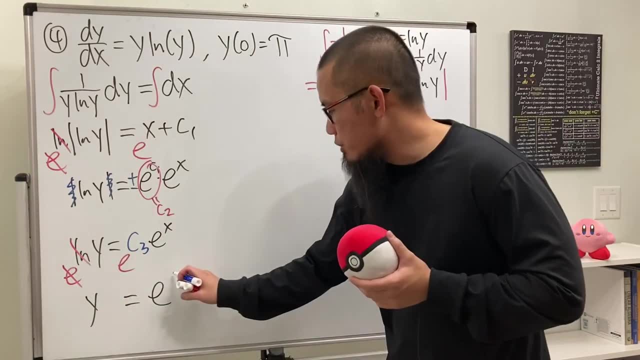 right hand side, we get e to that power, so i'm going to just write it down e. and then we have the c3, but the y is isolated, so i'm just going to put it down as c, and then we have e to the x power. 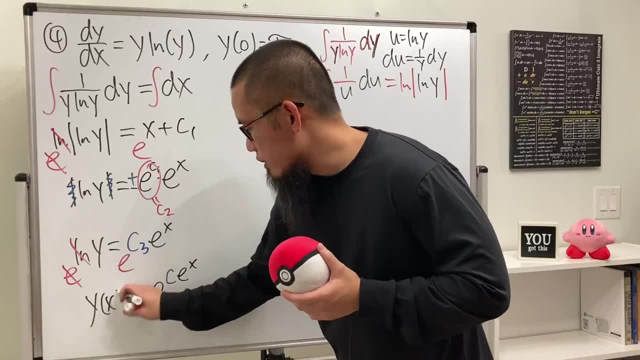 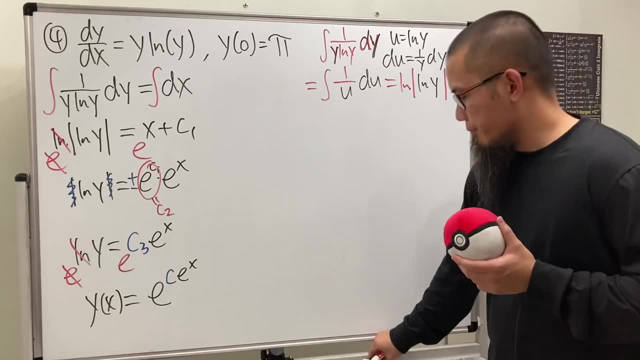 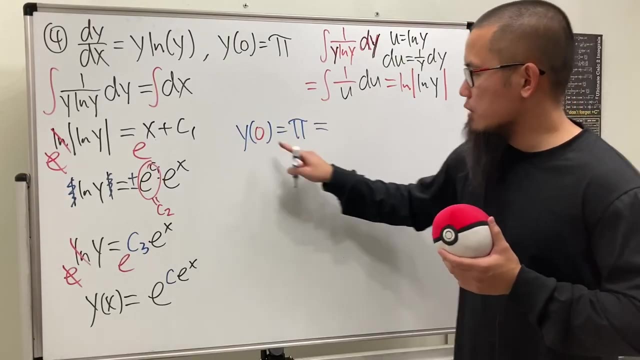 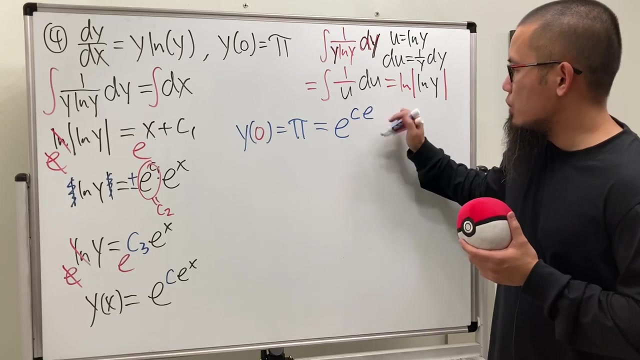 like that. okay, so y as a function of x. this right here is a general solution for for that. with that, though, we know y of zero equals pi, and uh, we'll just put a zero into this x here. so we are looking at e to the c times, e to the zero. this is pi. that's good. 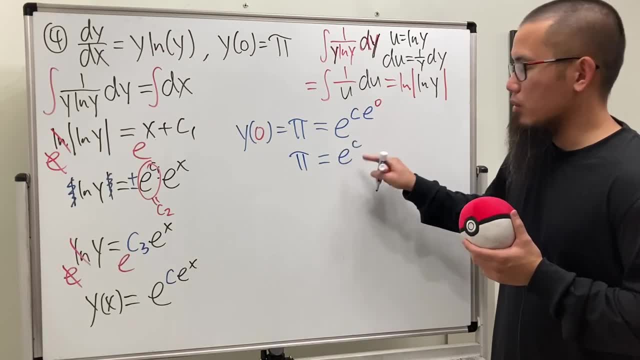 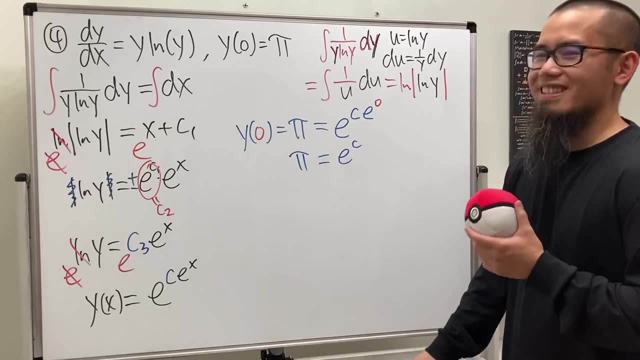 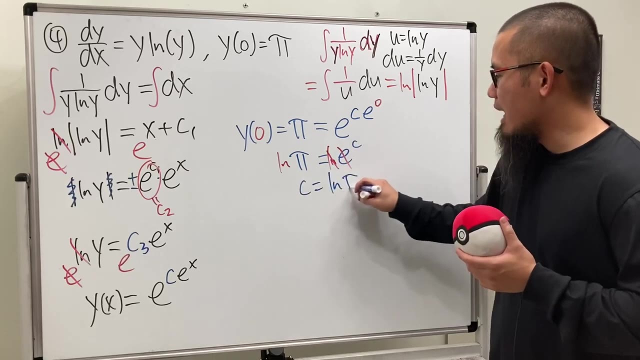 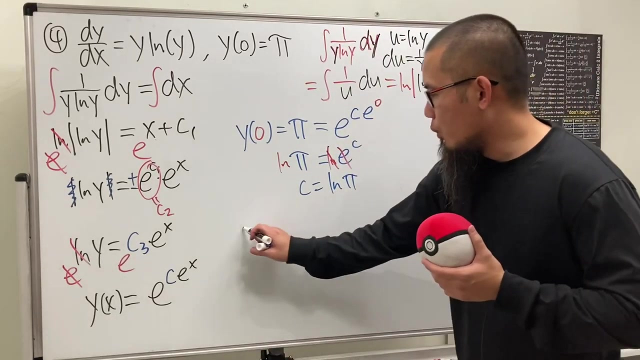 e to the zero is one, but look at this as e to the c, though, right here. wow, that was this. where's the number, this normal number? oh, my goodness, by the way, ln, both sides, so that we can get rid of this. so c is equal to ln pi. so we can put that down right here, ladies and gentlemen. y as a function of x. 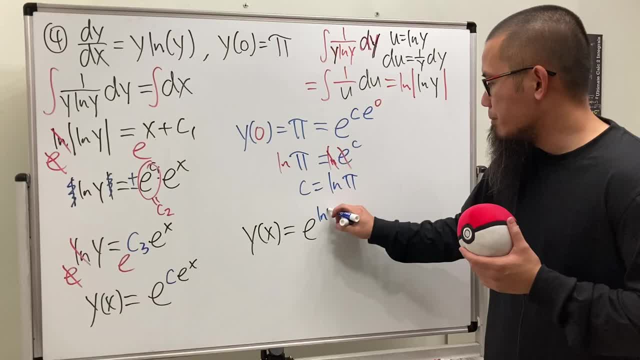 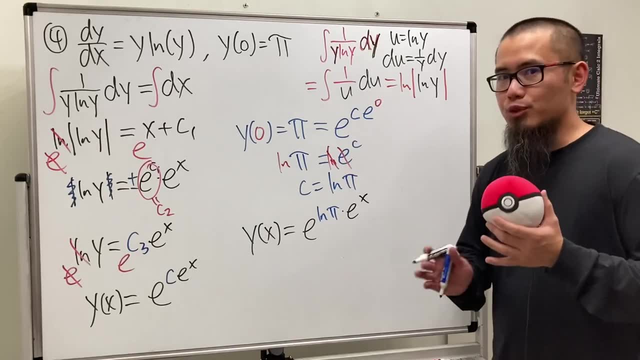 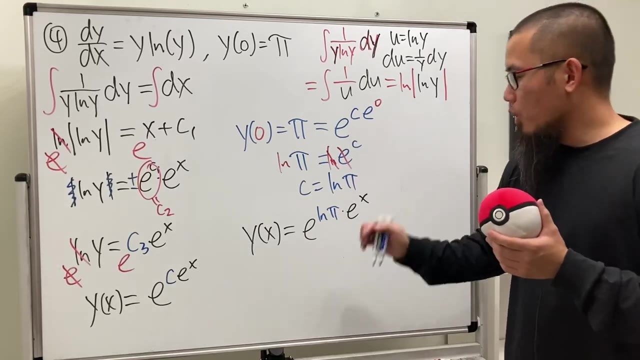 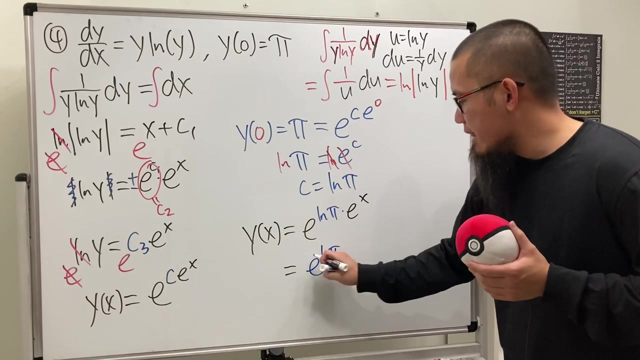 is equal to e. and then we have ln pi times e to the x power. you can just leave it like this, but i'm going to show you guys what's even cooler than this. so what's even cooler right here is that we can just- let's use the calculator. you can look here. okay, so u times e to the c is equal to the. 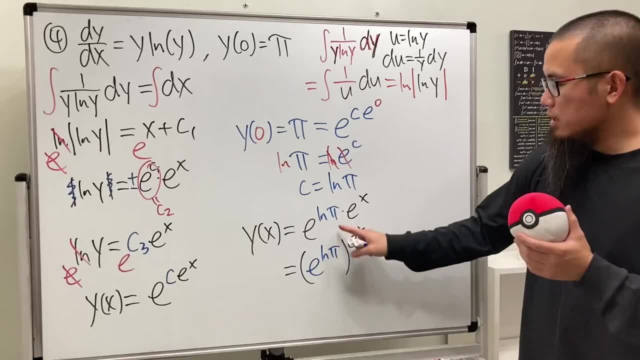 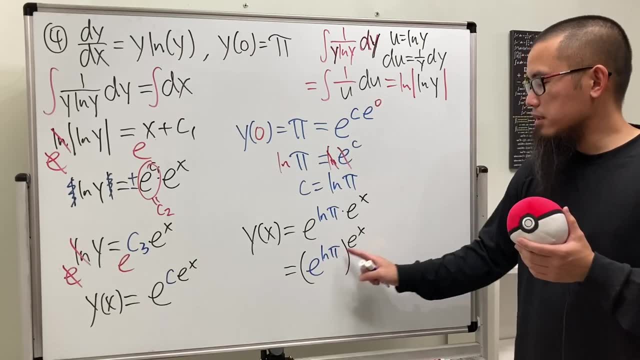 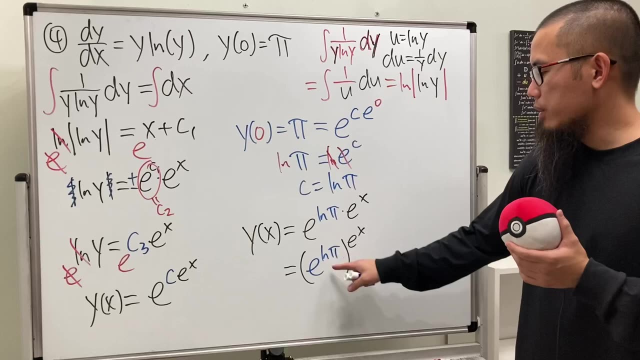 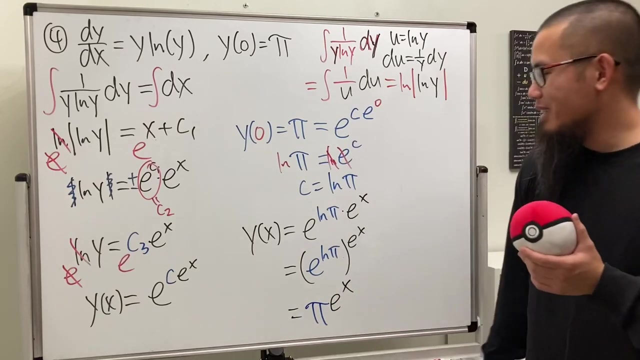 e to the z power. yeah, Congress conspiracy theory. yeah, my math isn't legal. yeah, when we come back, we just pick only the1, 2 when we connect both by 2, l and cancel, and you'll just end up with pi and then e and then to the x power. wow, that is the. 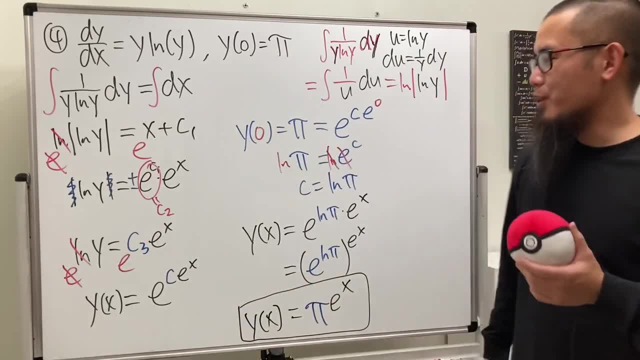 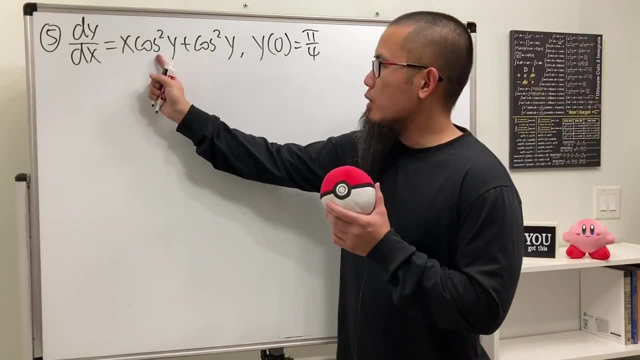 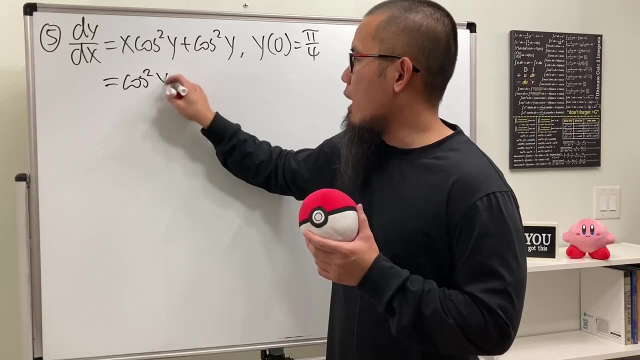 solution to that differential equation. with same initial condition, number five, dy dx is equal to all this. notice. we have cosine square y, cosine square y. we have to factor that out first. so that's going to make that happen. cosine square y and then times the rest will be just x plus one. 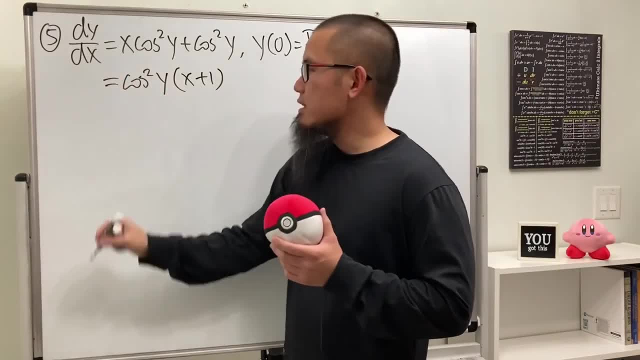 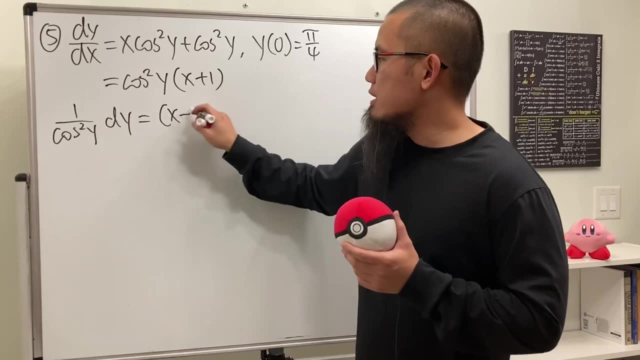 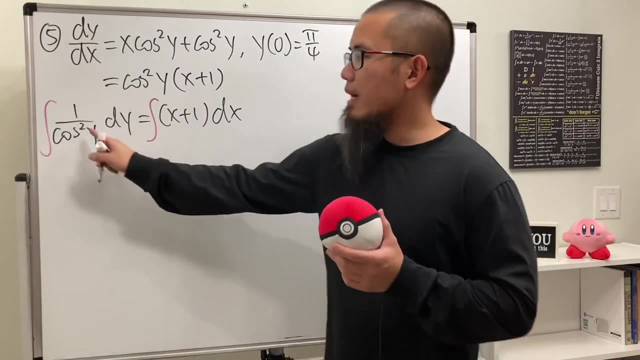 okay, divide this on both sides. so we get one over cosine square y with the dy here, and that's equal to parentheses x, plus one with the dx here. okay, this right here, integrate. this right here, integrate. but what's one over cosine square y, secant square y? so again, this right here. 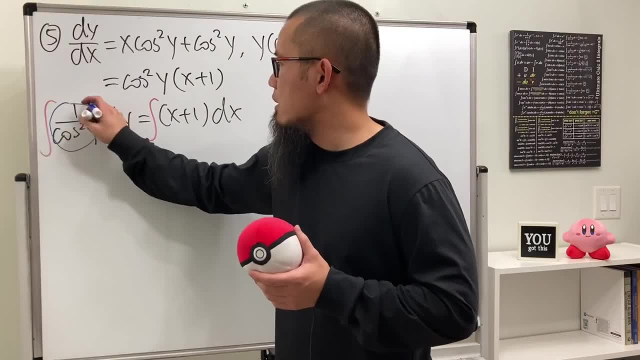 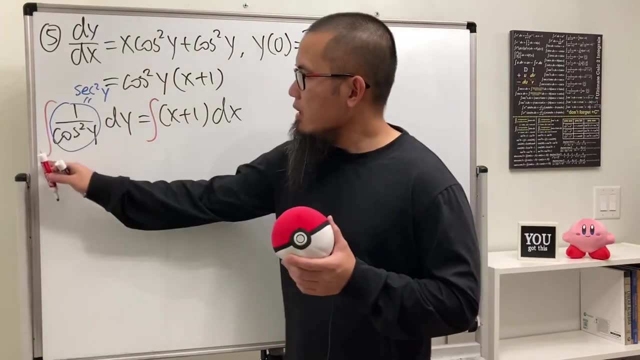 you can see that we have cosine square y and then times. the rest will be just x plus one is actually just secant. secant square y, right one over cosine secant, and then we have the second power. so when we integrate secant square, we get tangent. the left hand side give us tangent and 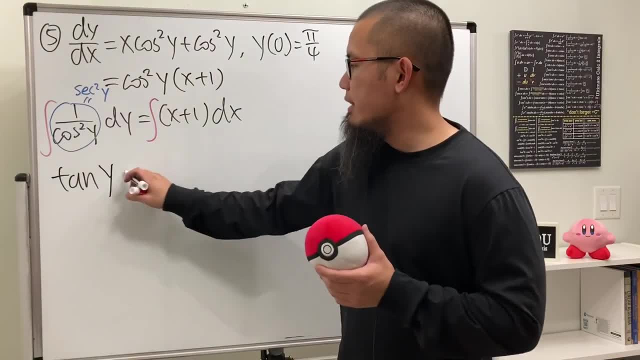 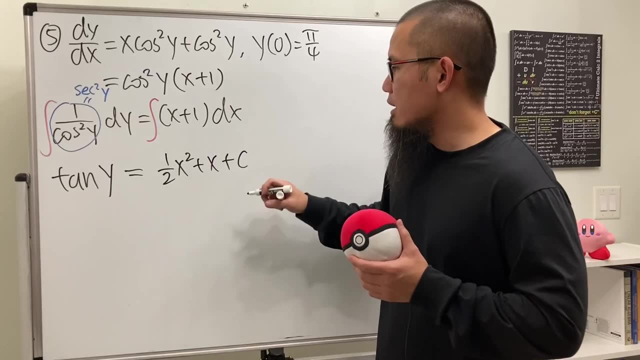 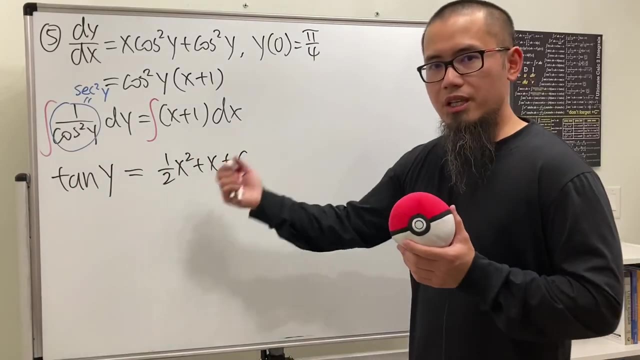 this is the regular tangent and the input is y, and then the right hand side. we get integral, this, which is one half x square plus x and plus c. c is enough. you'll see why. because i want to get the y by itself. we can just do the inverse tangent on both sides. 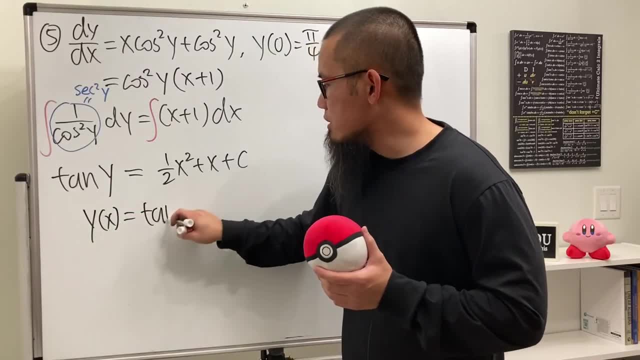 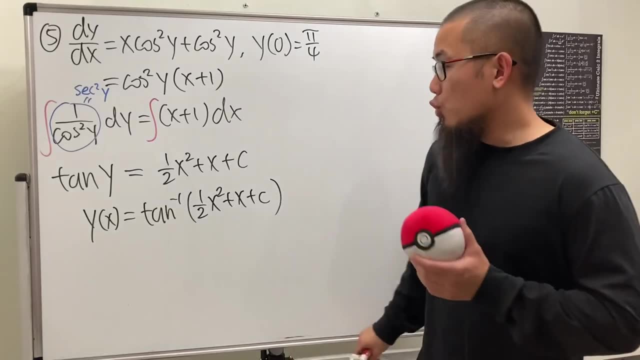 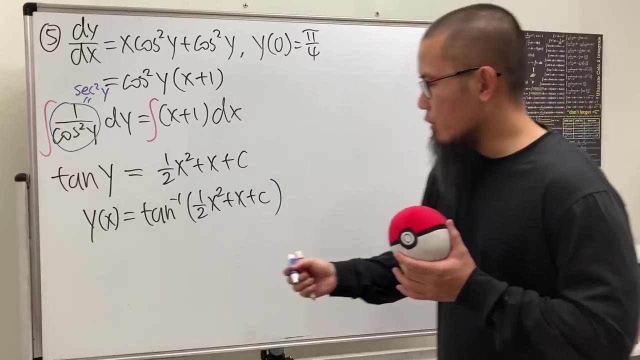 y as a function of x will just be inverse tangent of the entire right hand side, and that's one half x squared plus x plus c. cool, okay, y of zero is equal to pi over four. all right, so let's see: y of zero gives us pi over four, and then zero equal to pi over four. 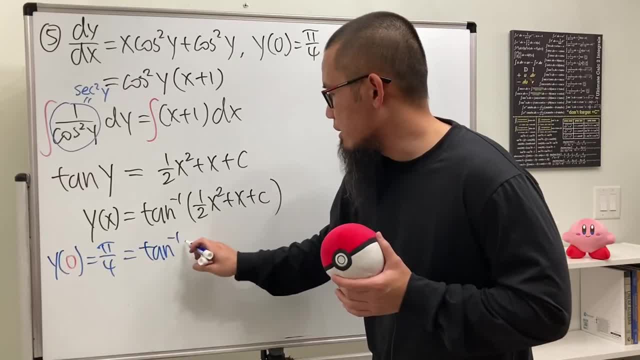 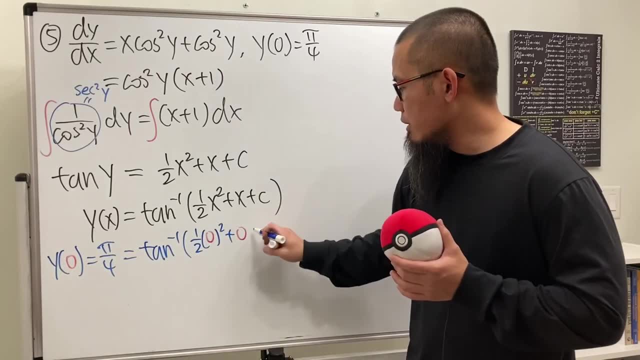 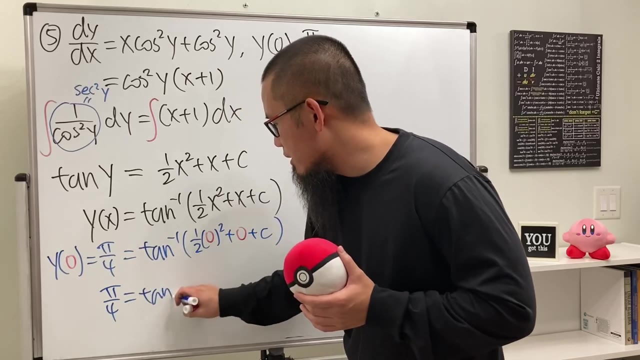 And we have inverse tangent of- and this is going to be 1 half x is 0, and then another x is 0, and then we have the c. So we are looking at pi over 4 equals inverse tangent of c. 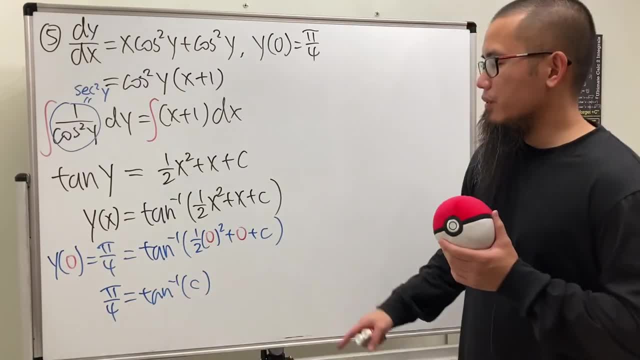 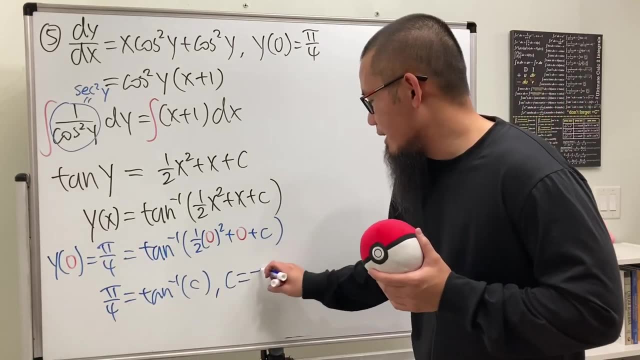 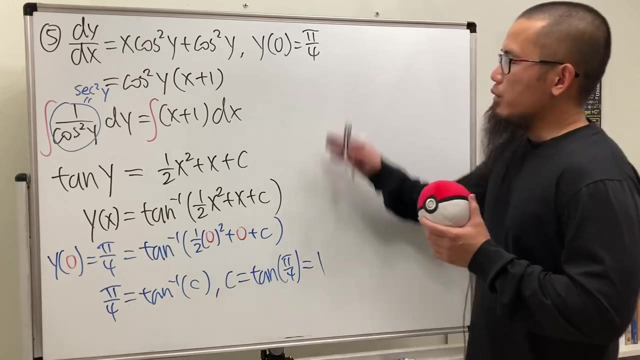 Okay, inverse tangent of pi will give you pi over 4.. You can look at this backwards, So c is just going to be tangent of pi over 4, which is just equal to 1.. Or, if you would like, you could have solved the c right here. 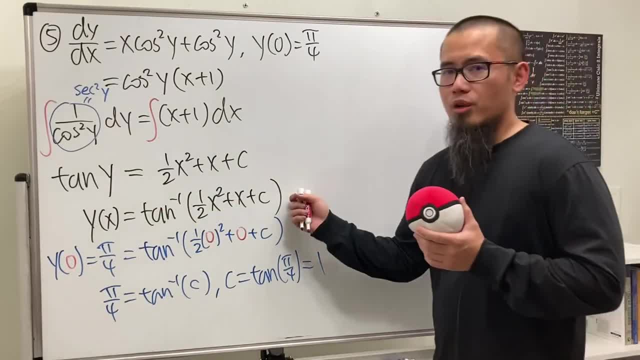 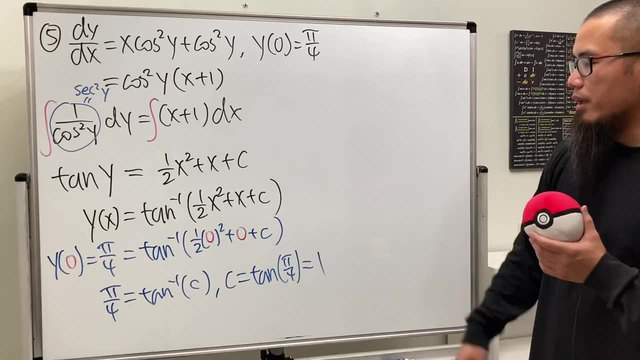 It might be easier, But I don't want to do it this way, because that way we can talk about the general solution, especially when we have the y-isolated. Okay, so we have: c is equal to 1, and now we can just write down the answer. 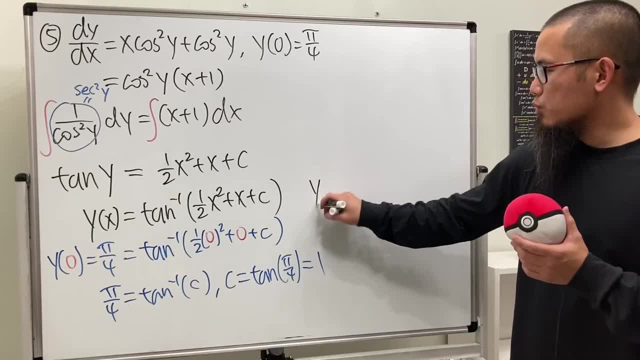 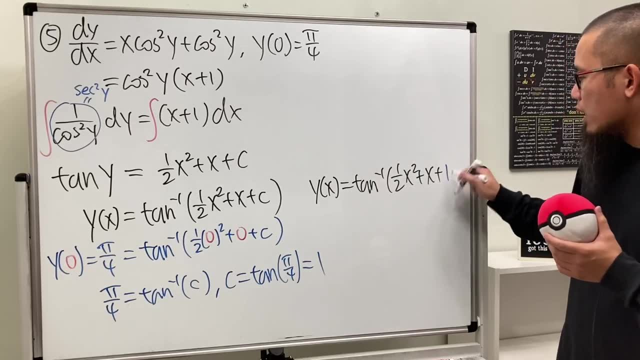 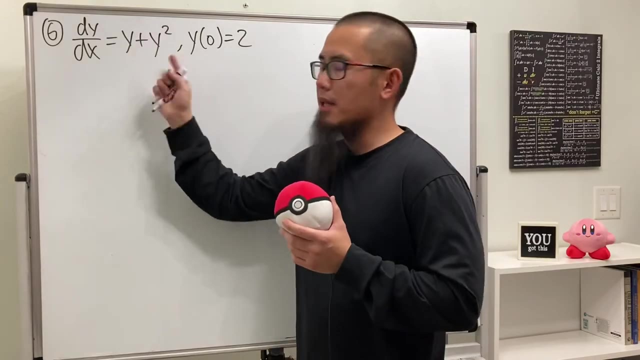 And, ladies and gentlemen, our answer is: y of n. x equals inverse tangent of 1 half x squared plus x plus 1.. Done Okay, number 6.. D, y, dx is equal to y plus y squared. Of course, we will have to bring both of them to the other side by dividing. 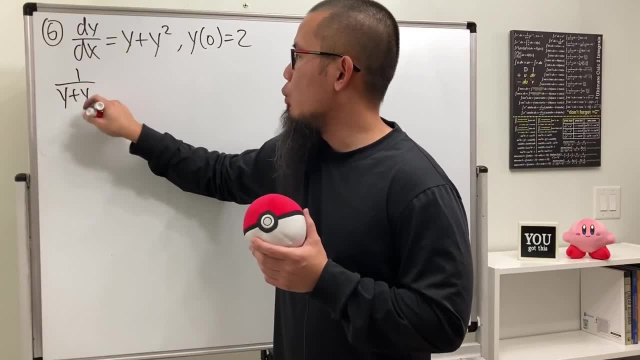 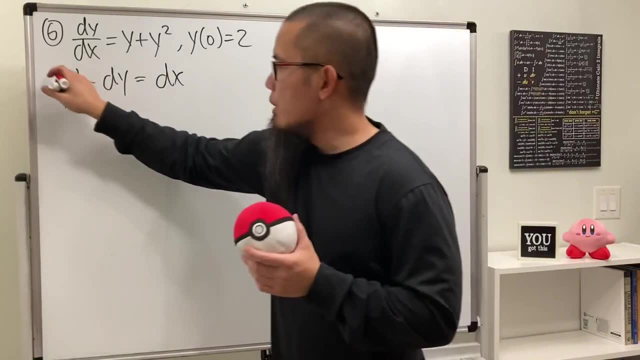 So we get 1 over y plus y squared, and then we have the dy here and we will just multiply the dx, right here. That's what we have. Integrate both sides, right. But how do we integrate this Notice on the bottom? we can actually factor it. 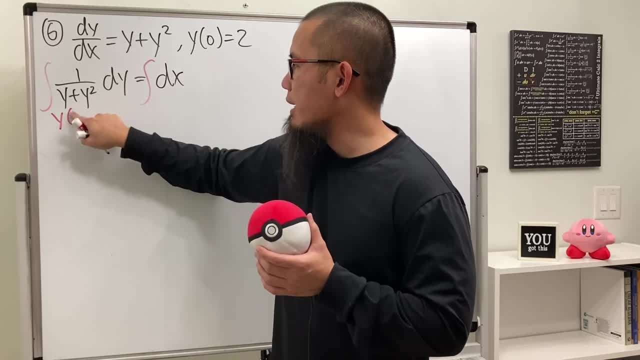 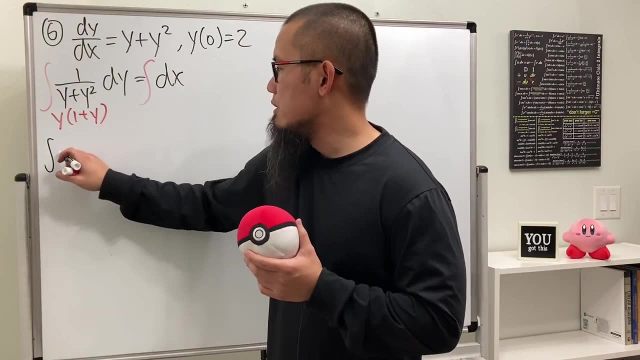 So when we do that we get y times 1 plus y, So we do partial fractions, Yes. So right here we are looking at the integral of some number over y plus some other number over 1 plus y. 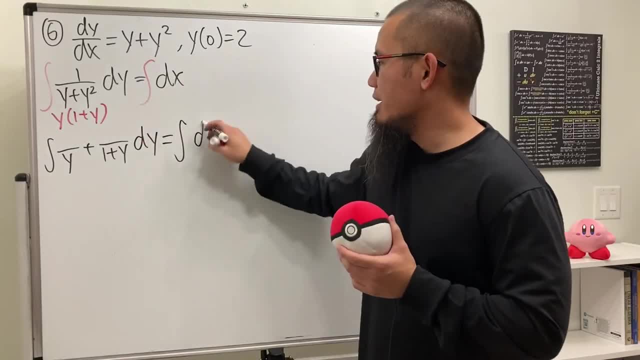 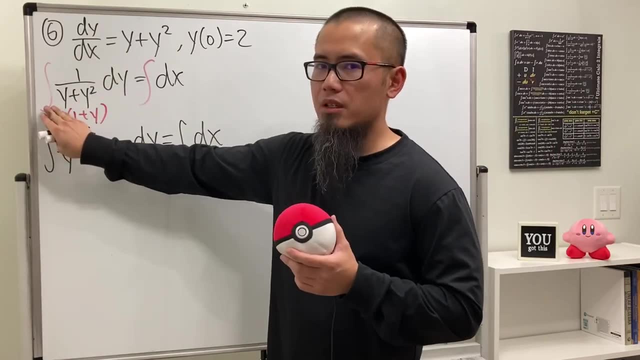 And then we are in the y world, And perhaps let me just leave the integral right here. on the other hand side too, To figure out this number, we go back to the original And cover the same denominator. How can we make y equal to 0?? 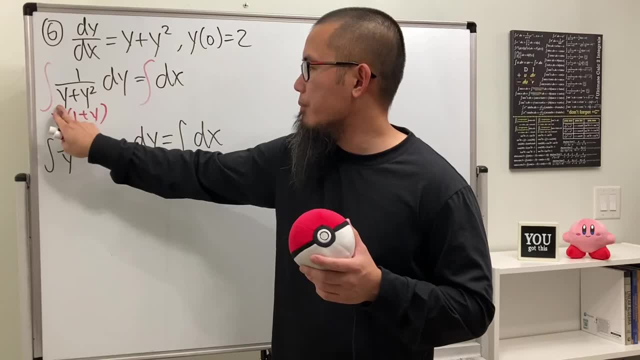 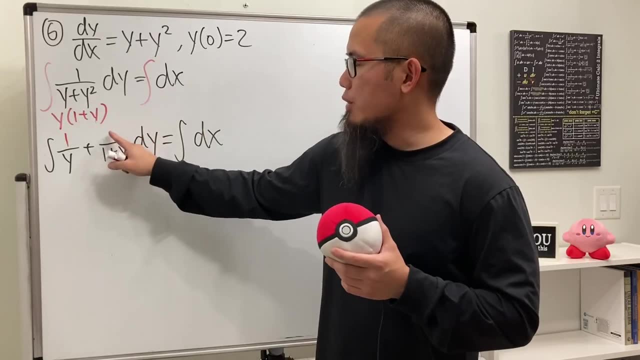 y has to be 0. And we put 0 into this y here And we get 1 over 1 plus 0, which is just 1.. Good, Now look at this right here. To get this right here: we cover the same denominator. 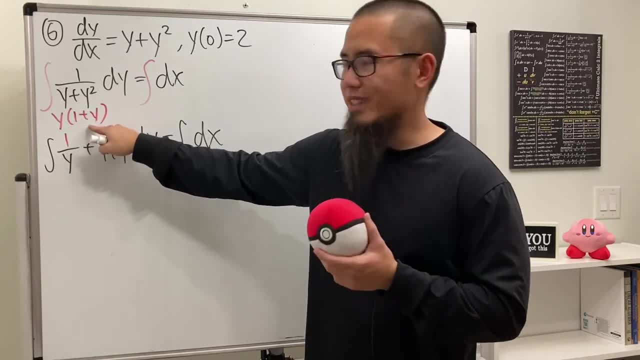 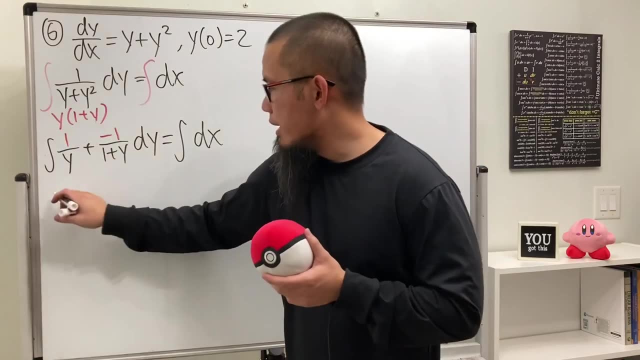 And how can we get this equal to 0?? y has to be negative 1.. Put it here: 1 over negative 1, we get negative 1.. Great, So integrate. now We get ln. Ln- absolute value of y. 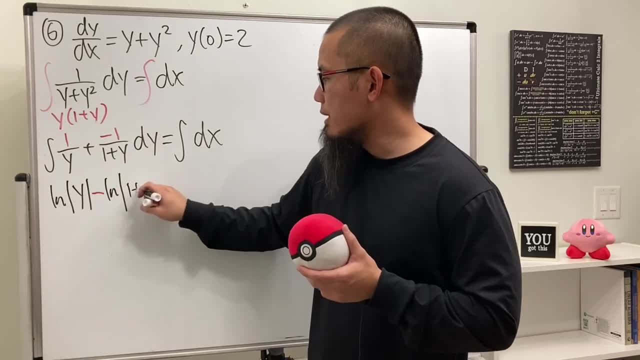 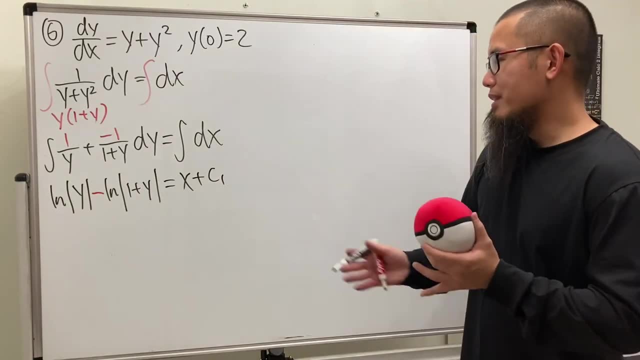 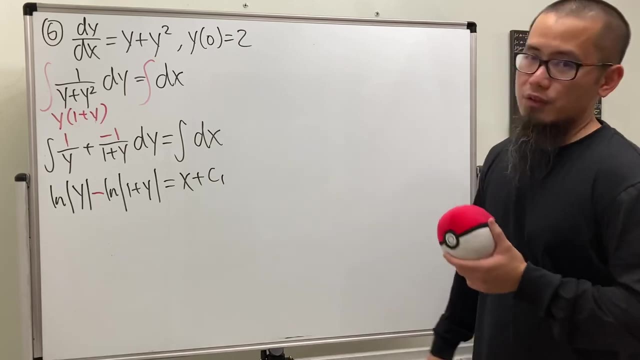 And then minus ln absolute value of 1 plus y, And that's equal to x plus c1.. Cool, So we are done with the integration, And then the rest is just algebra, And let's just go ahead and solve for y. 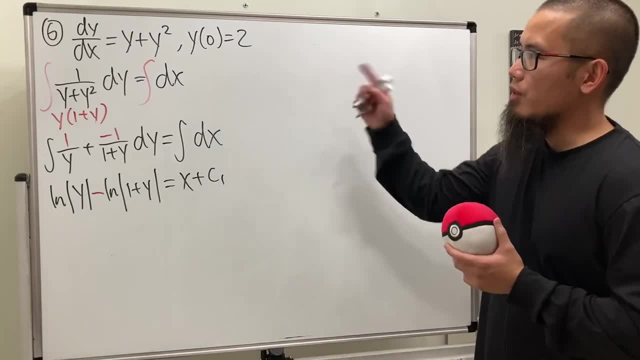 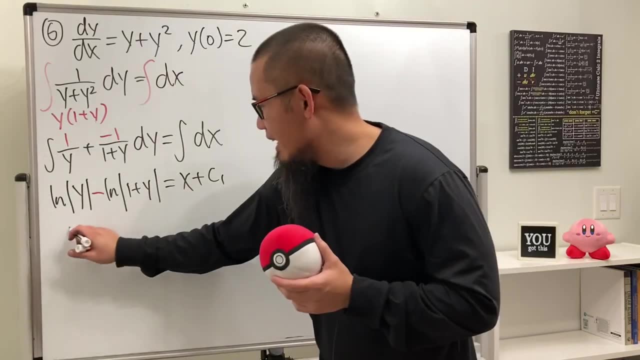 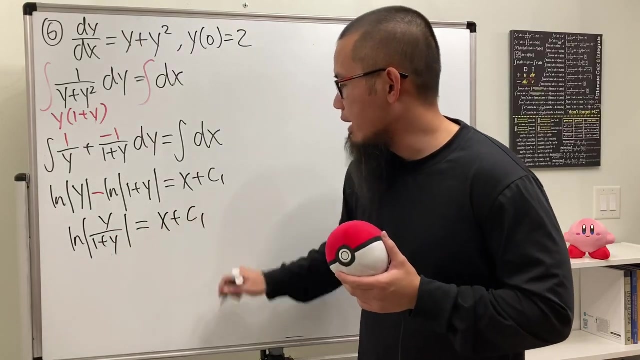 Because again I want to look at the general solution first, before we solve for the constant. So to get that happen we are going to combine logarithms first. So we get ln, absolute value, this over that y over 1 plus y, and that's equal to x plus c1, and 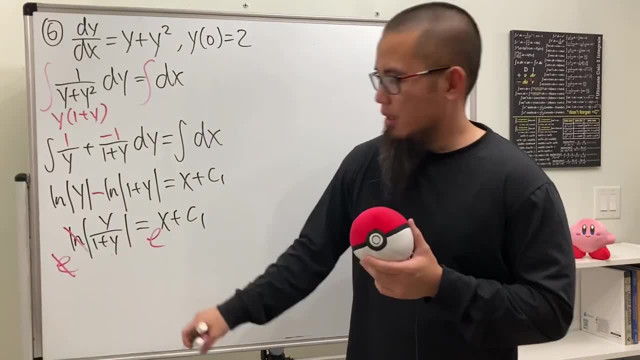 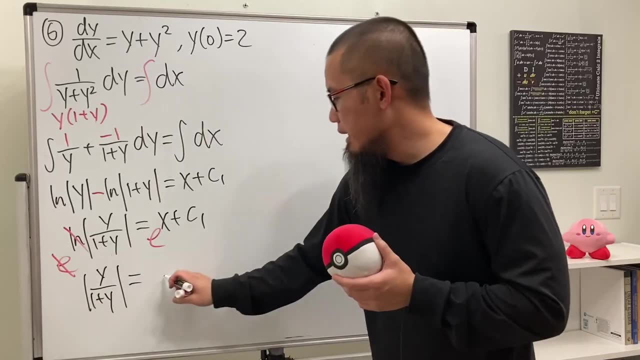 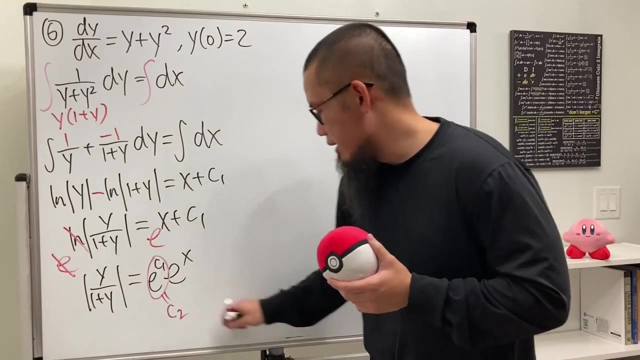 then do e to that power, e to that power, cancel this out. so we get absolute value of y over 1 plus y equals e to the x and then times e to the c1. This, right here again, is just c2.. 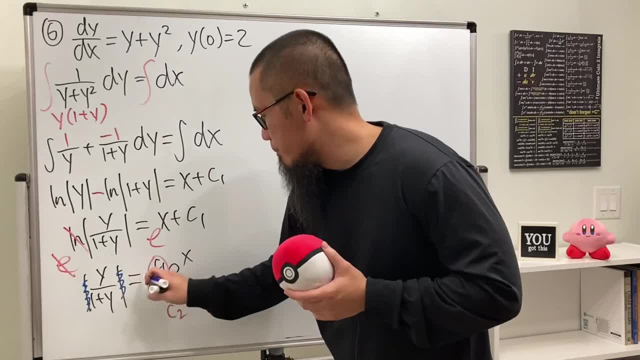 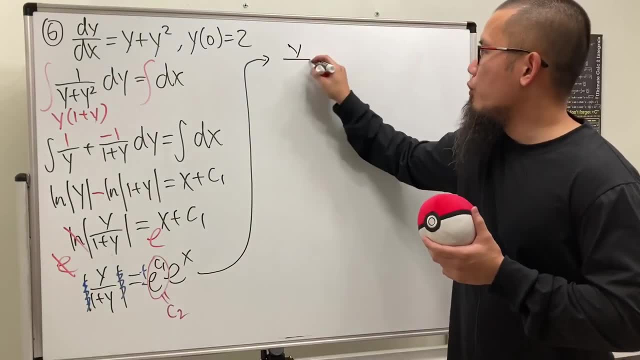 And then get rid of the absolute value. Put the plus over here, Put the plus over here, Put the plus or minus, like the good old business, draw a big arrow and then the left-hand side is that y over 1 plus y, and that will be equal to. you know the deal, that little. 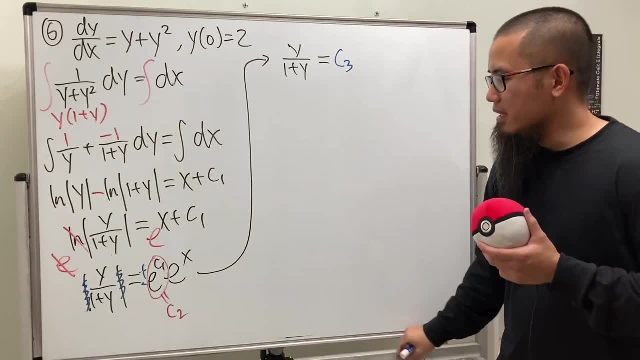 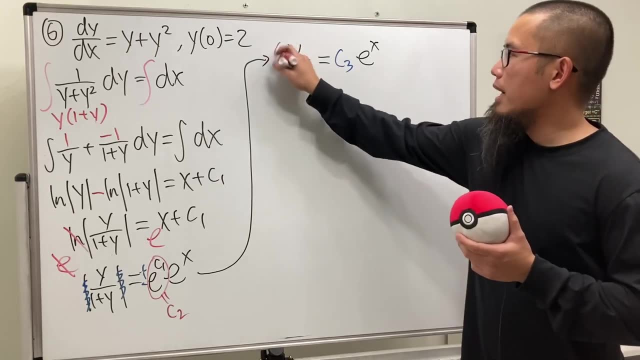 things together is just c3,. and then we have e to the x power. Very nice, Now to get the y by itself. let's multiply this equation by the denominator, which is just 1 plus y, And we will get y. 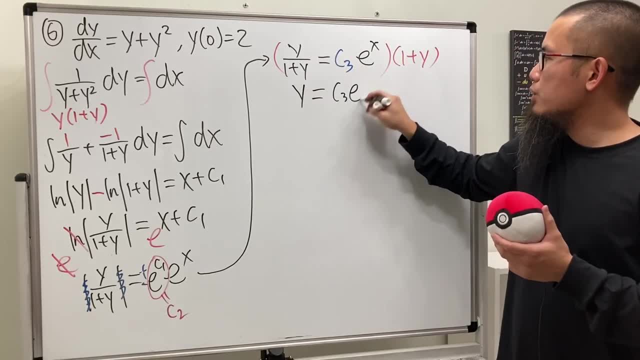 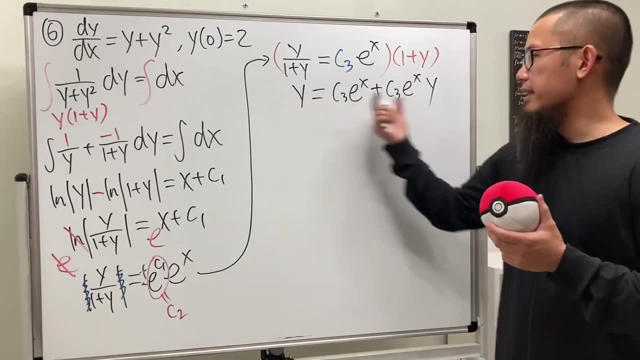 e to the x power. e to the x power equals distribute. we get c3e to the x times 1, and then this times that. so plus c3e to the x and then y Notice this and that they both have the y. 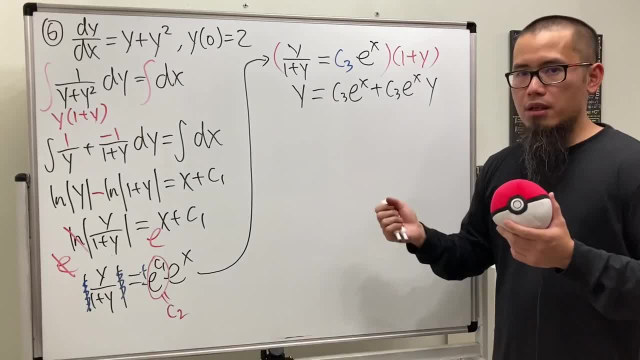 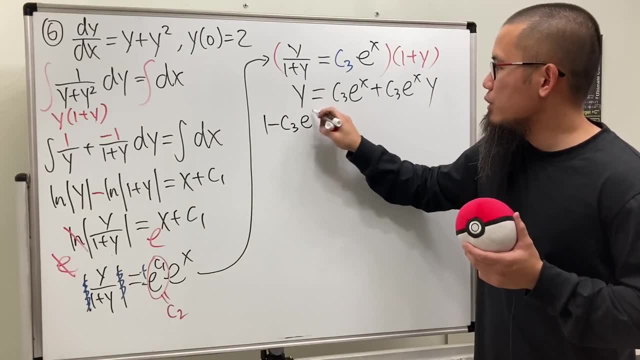 I'm going to bring this to the left-hand side and then factor out the y. The coefficient right here is 1, and then, once we bring this to the other side, we will have minus c3e to the x, and then we'll factor out the y and put it at the end. 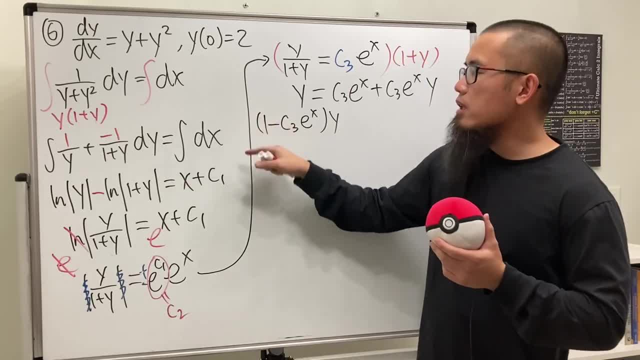 I recommend you guys to put this at the end, because if you put the y at the end, you're going to get c3e to the x. If you put the y in the front, it looks like y as a function of that, but that's not what. 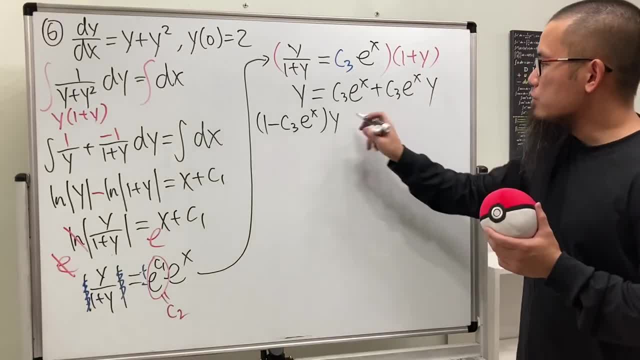 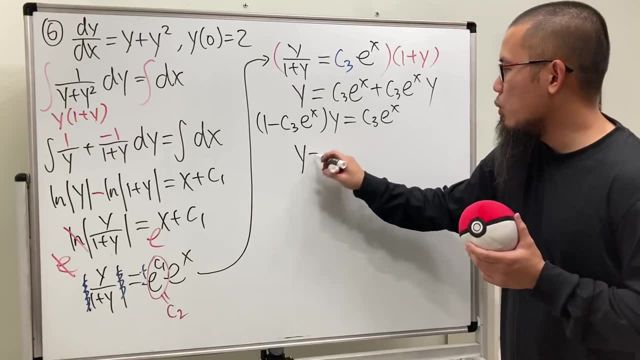 we're talking about. so this is a better form And this right here is equal to c3e to the x. In the end we can just divide this on both sides, so we get y equals c3e to the x over. 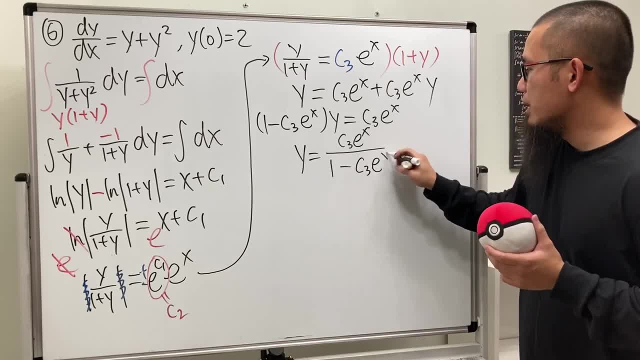 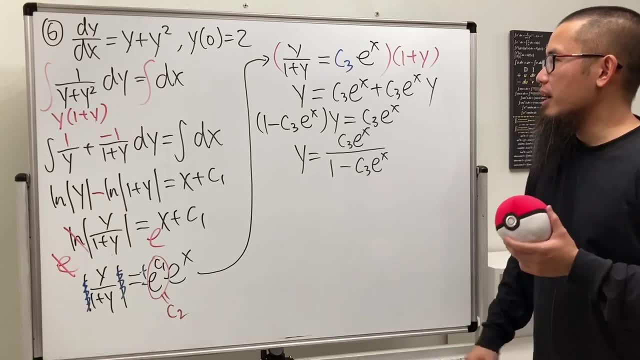 1 minus c3e to the x. Yeah, just like that. Now it's totally okay if you just stop right here and then just go ahead and figure out how to plug in 0 for x and y for 2, and then solve for c3. 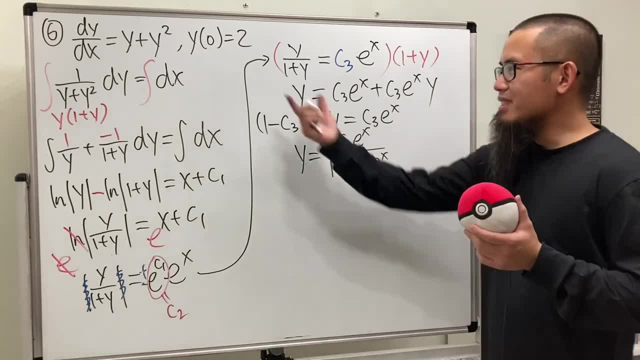 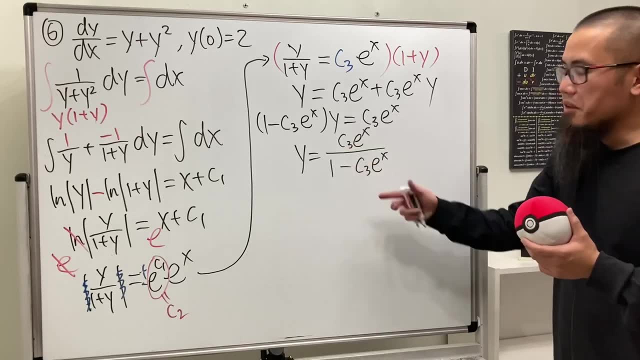 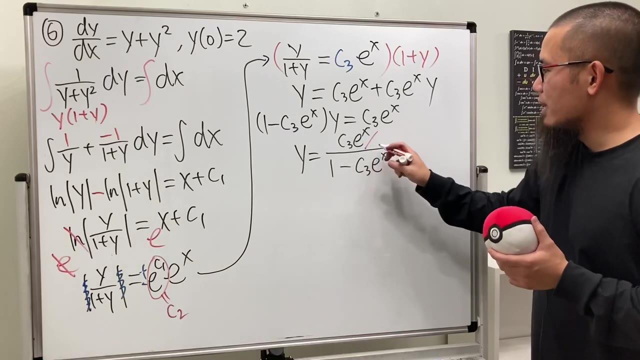 However, this is what we usually do, because this right here is actually a simplified version of a logistic differential equation. You'll see that this and that are the same right, So we're actually going to divide this for the whole thing. so divide this by c3e to: 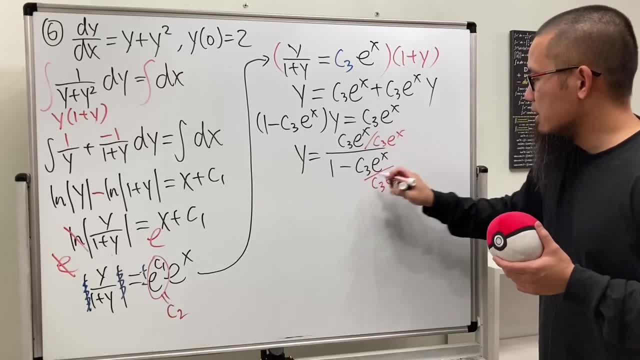 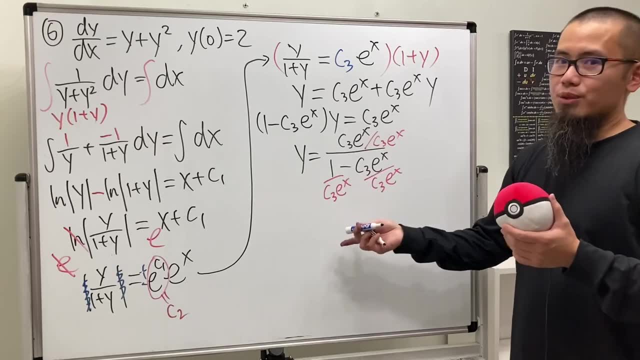 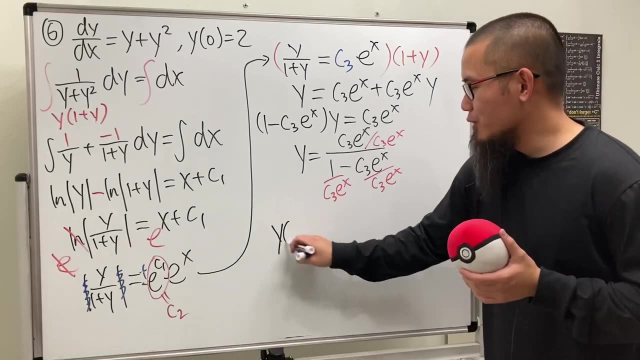 the x and then divide this by c3e to the x and then also divide this by c3e to the x. This way you can see that we just have to deal with the constant at one place. This right here is y, and then I'm finally done so. I'm just going to put down y as a. 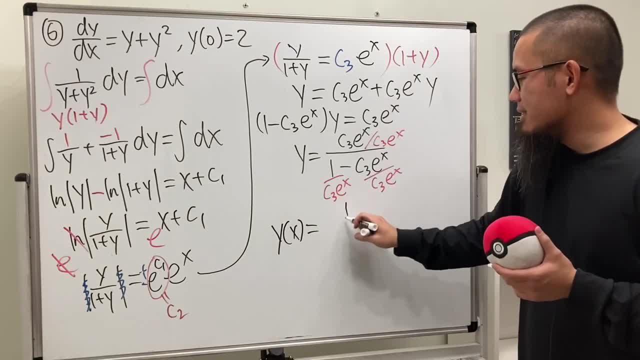 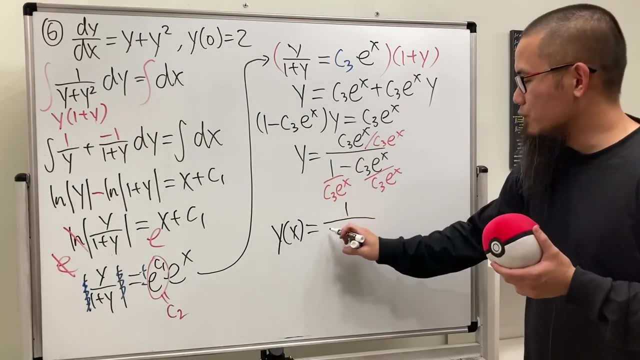 function of x. On the top it's nicely equal to just 1.. Check this out: 1 over c3 is another constant right, Which is just c4, but we're all done so I'm just going to put it as c, like this normal. 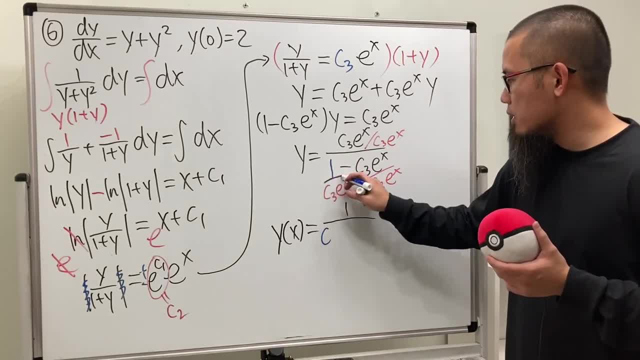 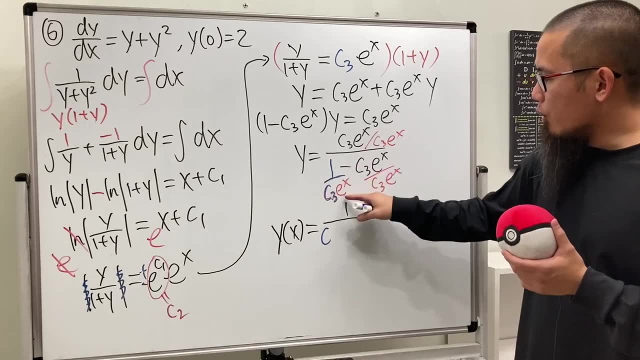 operation. we'll do So. 1 over c3, which is technically c4,, but we don't need a subscript anymore. However. 1 over e to the x, which is just the same as e to the negative x, and then. 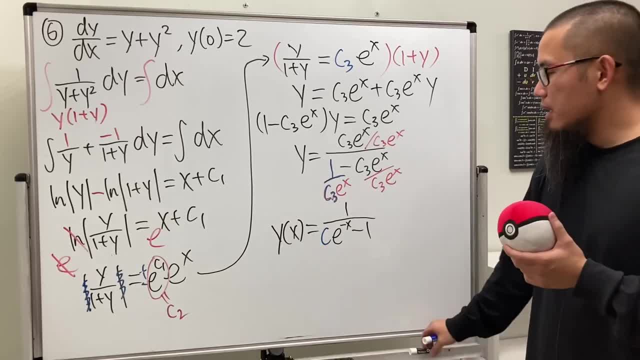 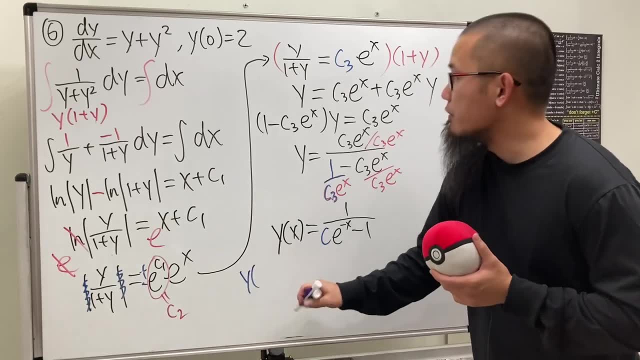 this is just going to be minus 1, so that's what we have Good. Now we'll use the initial condition to solve for the c. We know y of 0 is equal to 2, which is 1 over c3.. 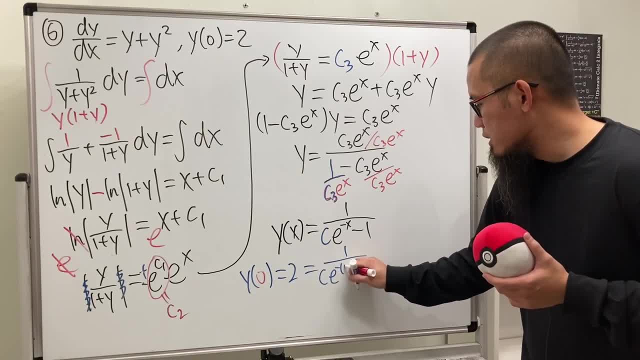 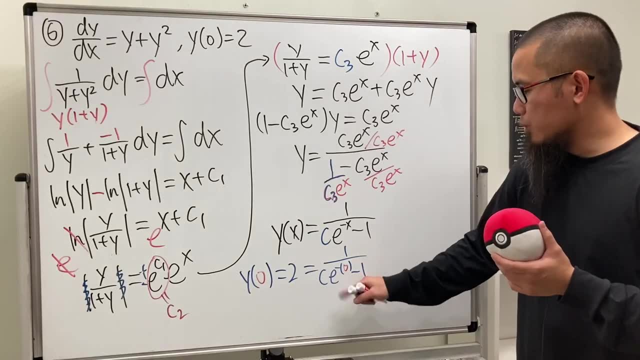 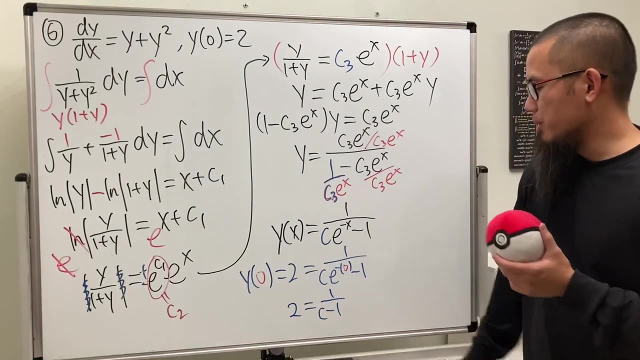 c e raised to a negative 0, and then minus 1.. Check this out: This is going to be just 1, so we just have 2 equals 1 over c minus 1, and then you can just think about what c should be. but if you would like, you can multiply the c minus. 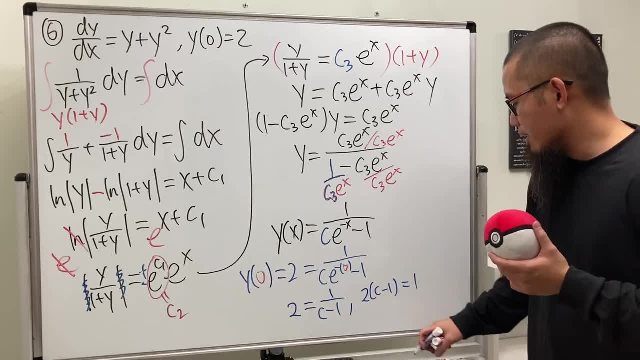 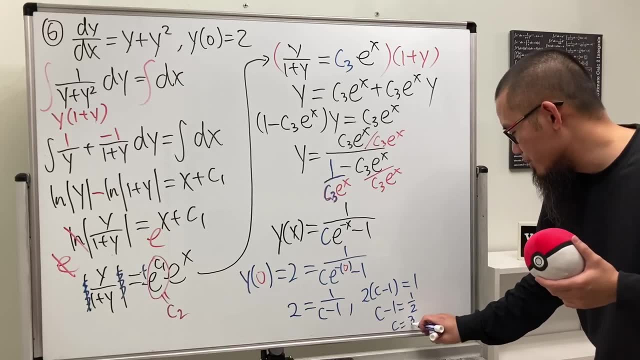 1 on both sides. so 2c minus 1 is equal to 1.. Just do your business. And then c minus 1 is equal to 1 half, And then c is equal to 3 over 2, right.